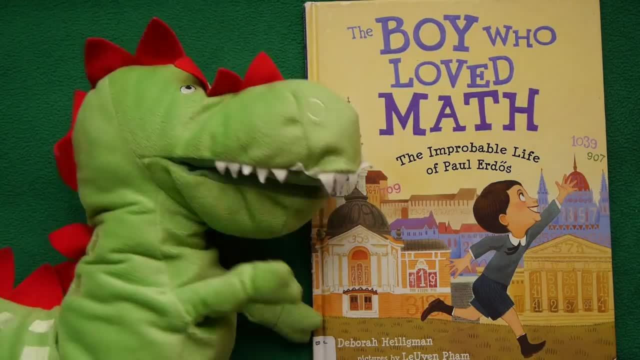 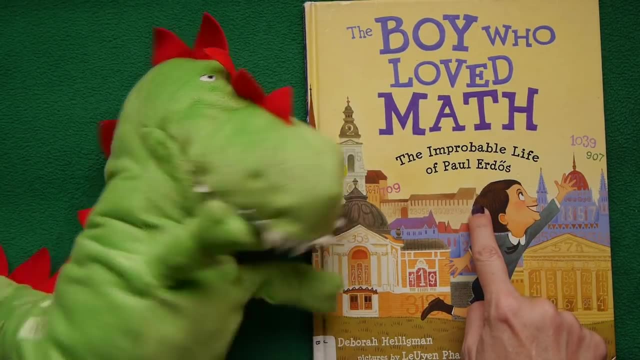 I've never heard of him. And how does one become the most incredible mathematician of time? Well, let's find out. Oh, you're going to show us from when he was a little boy. Oh, I love these stories, Okay, okay. 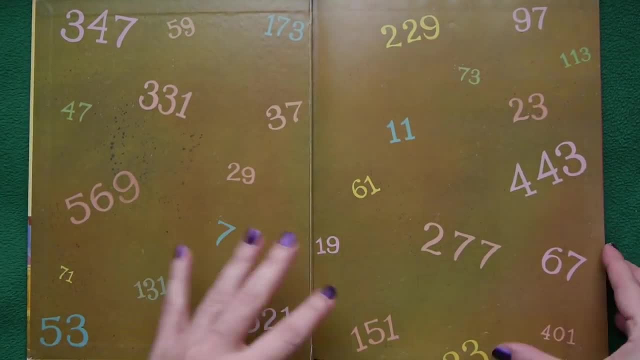 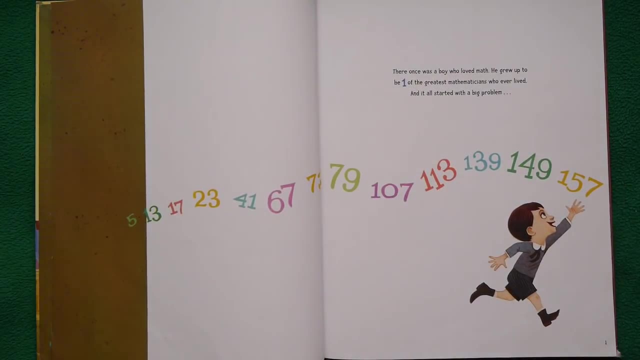 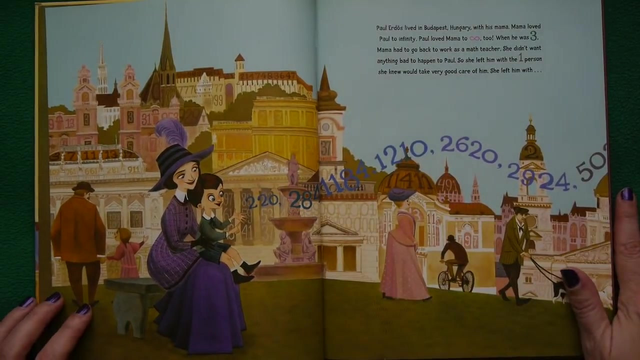 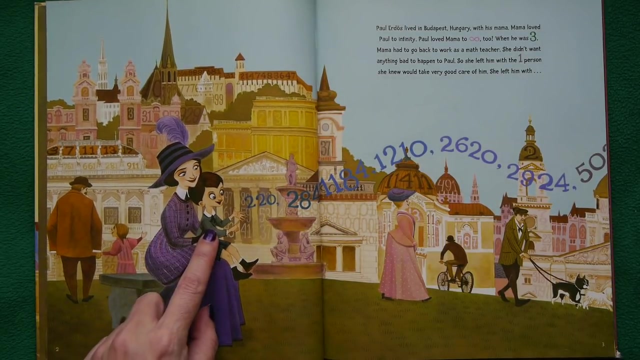 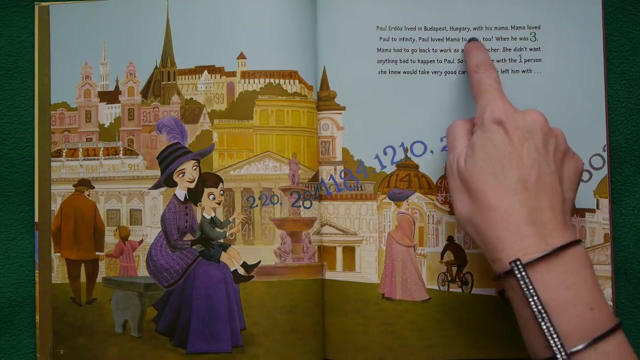 All right, let's see. How did a simple boy from Hungary become one of the greatest mathematicians of all time? There once was a boy who loved math. Well, that's simple enough. That's a good way to start. He grew up to be one of the greatest mathematicians who ever lived, And it all started with a big problem. Literally probably. Paul Erdish lived in Budapest, Hungary, with his mama. Mama loved Paul to infinity. Mama loved to what- To also make math too. 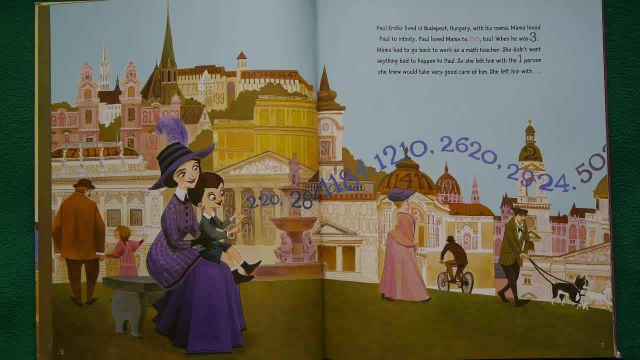 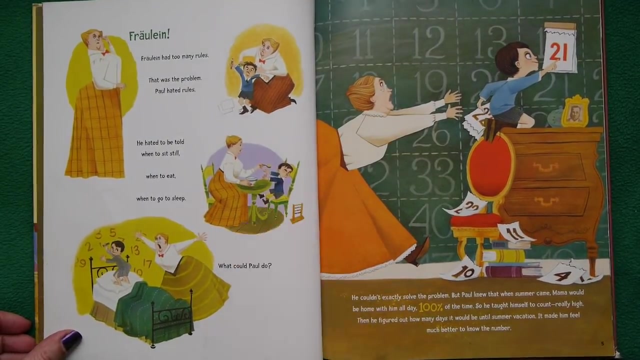 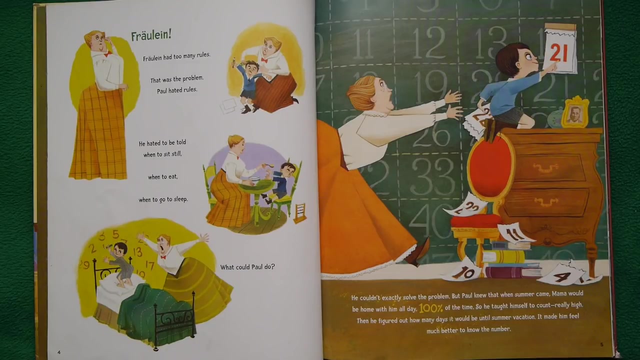 Mama had to go back to work as a math teacher. She didn't want anything bad to happen to Paul, so she left him with the one person she knew who would take very good care of him. Okay, She left Paul with Fraulein. Uh-oh, Fraulein had too many rules. There was a problem. Paul hated rules. He hated to be told when to sit still, when to eat, when to go to sleep. 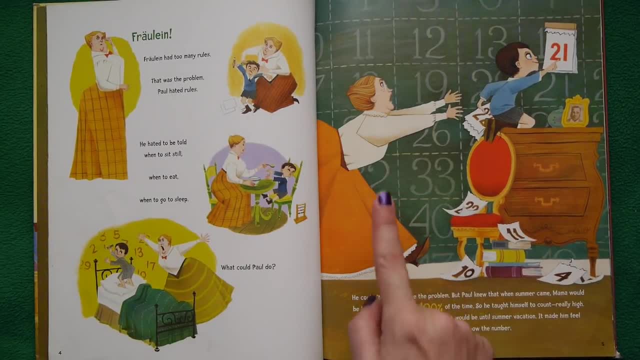 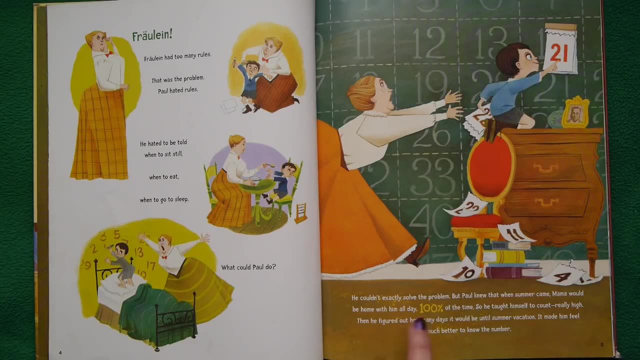 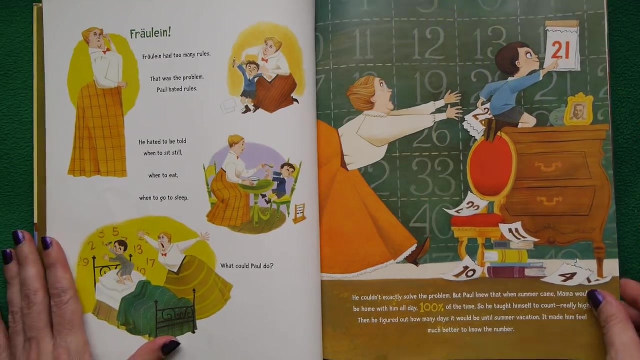 What could Paul do? Well, he couldn't exactly solve the problem of Fraulein, but Paul knew that when summer came, mama would be home with him all day, 100% of the time. So he taught himself to count really high. Then he figured out how many days it would be until summer vacation. It made him feel much better to know the number. Oh, that's something you could try. 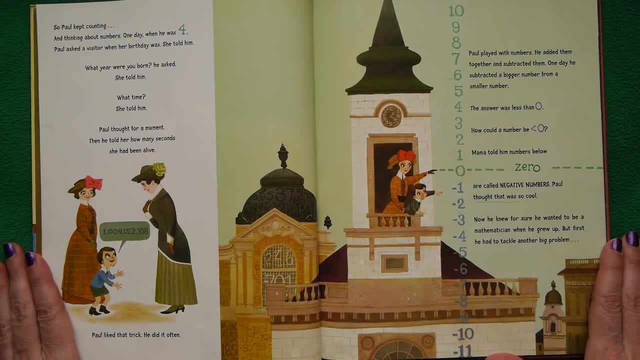 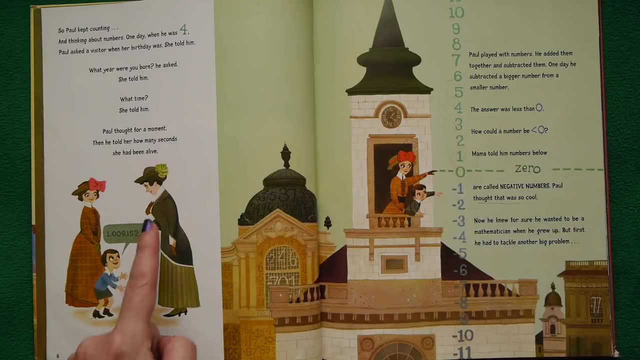 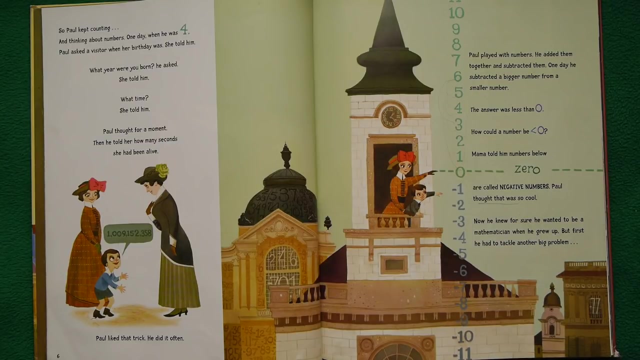 Okay, He started thinking about numbers. One day when he was four. Paul asked a visitor when her birthday was. So she told him: What year were you born? He asked. She told him What time. She told him. Paul thought for a moment. Then he told her how many seconds she had been alive: 1,900,152,358. 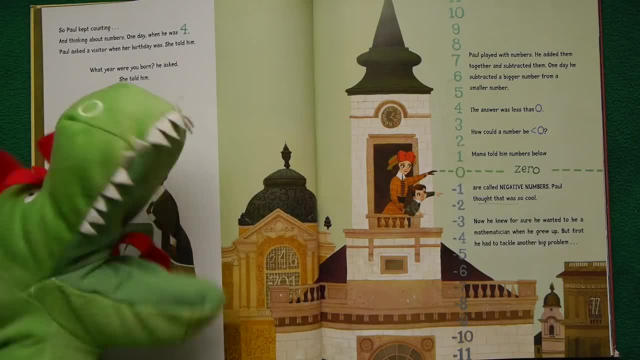 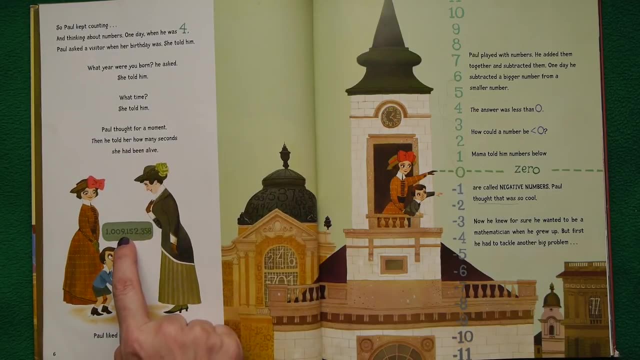 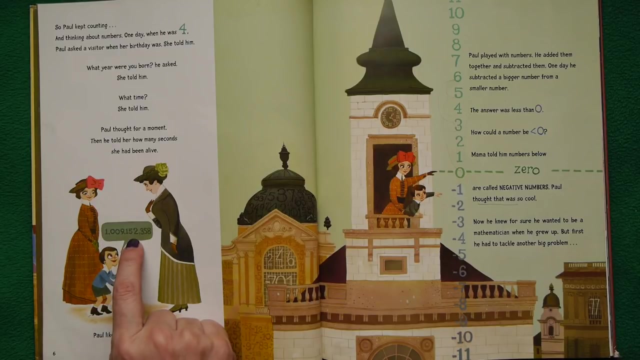 Wow, Just wow. Paul liked that trick. He did it often. That is an amazing trick. So she had been alive. Let's see 1 billion. I misspoke 1 billion 9 million 152,358.. 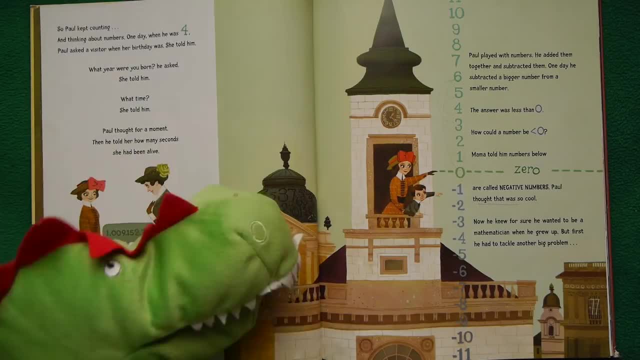 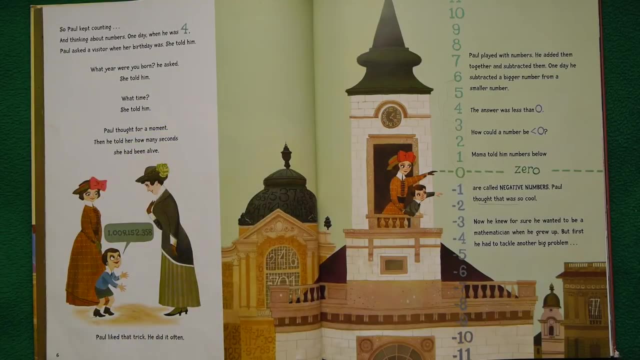 Wow, He calculated to a billion, just like that. That is a math genius, Yes, Well, Paul played with numbers, which is very good, You're a numbers guy. He added them together, subtracted them. One day he subtracted a bigger number from a smaller number. 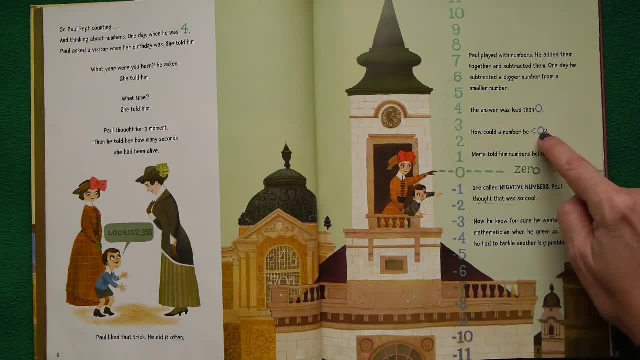 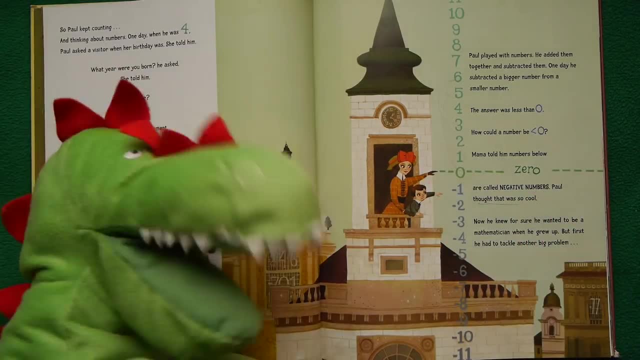 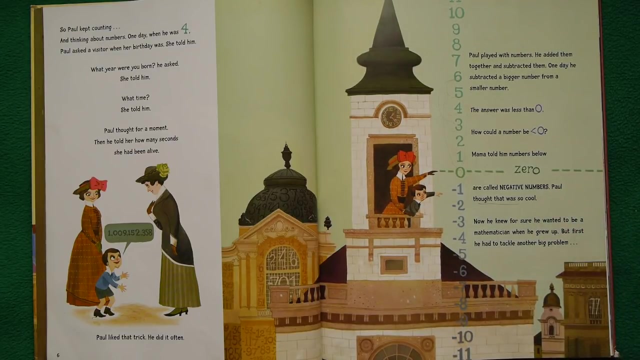 The number was less than zero. How could a number be less than zero? Mama told him, the numbers below zero are called negative numbers. I've got to write this down. See, Paul thought that was so cool, the idea of negative numbers. Now he knew for sure. he wanted to be a mathematician when he grew up. 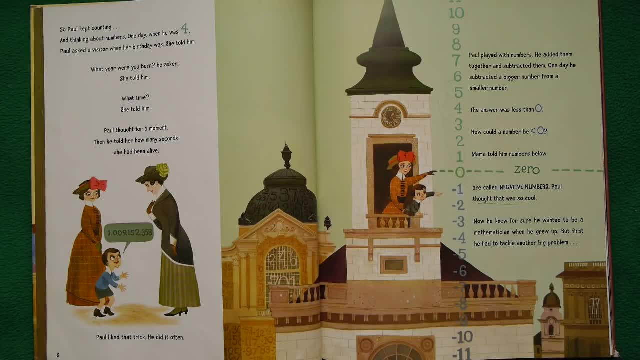 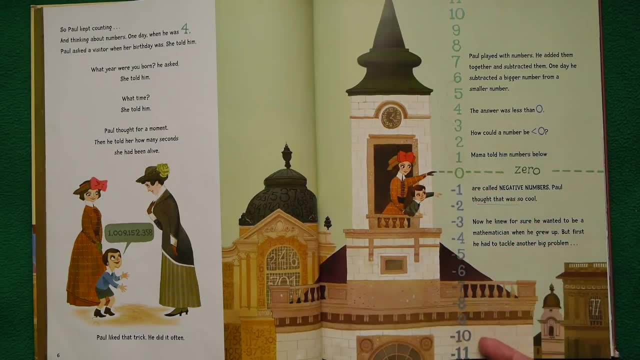 But first he had to tackle another big problem. But wait, Let's look, They're below zero. Now we get into negative one, negative two, negative three, four, five. It's all the same numbers, but going in the opposite direction. 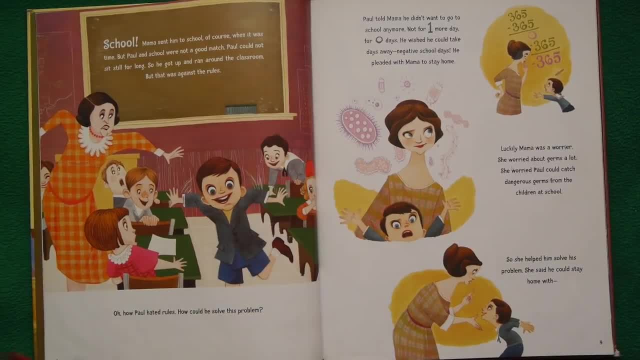 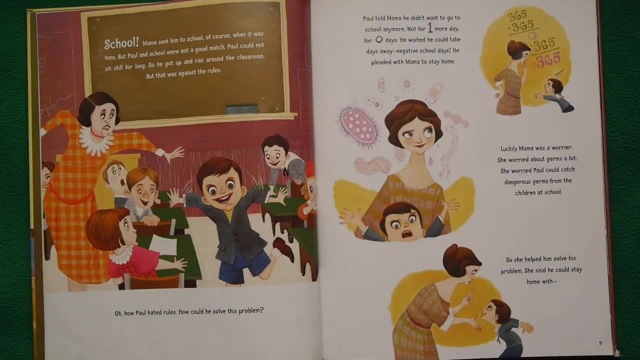 So what is this other big problem? School. Okay, this is gonna get interesting. Yes, Mama sent him to school, of course, when it was time, but Paul and school were not a good match. Paul could not sit still for long, so he got up and ran around the classroom. 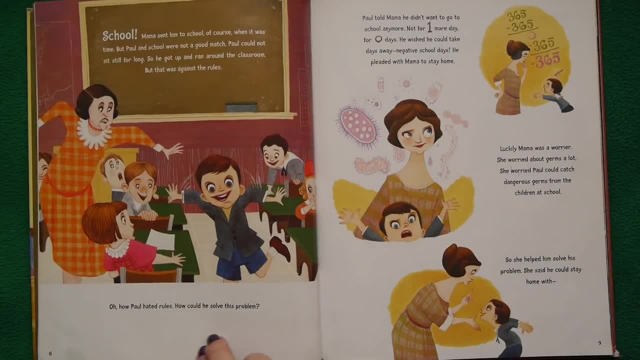 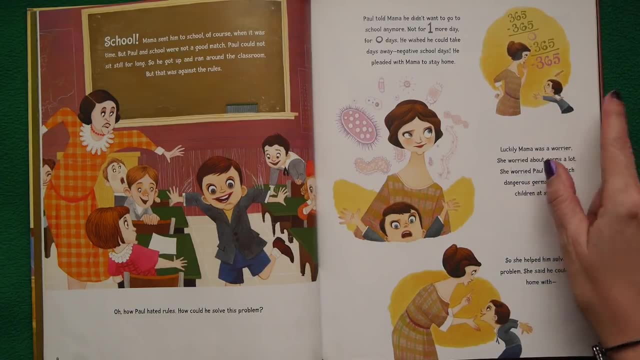 Bye. But of course that was against the rules. Oh, and you know how Paul hates rules. How could he solve this problem? Well, Paul told Mama he did not want to go to school anymore, Not for one more day, For zero days. 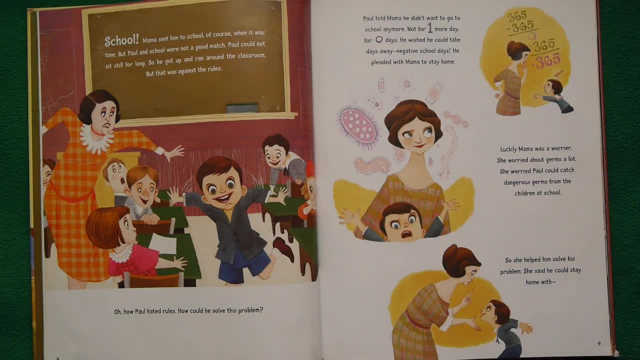 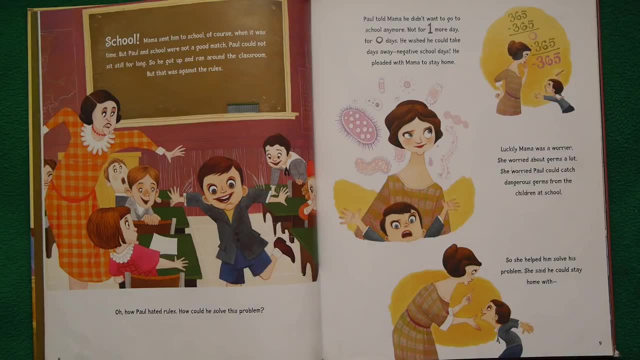 He wished he could take days away, Negative school days. He pleaded with Mama to stay home. Luckily, Mama was a worrier. She worried about germs a lot. She worried Paul could catch dangerous germs from the children at school. Oh, 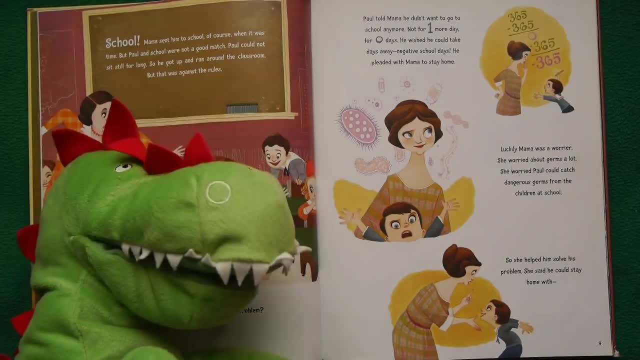 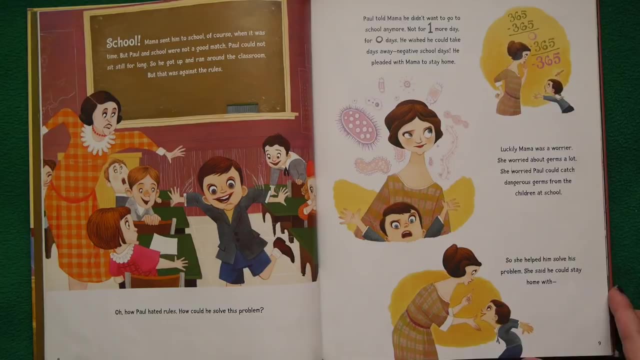 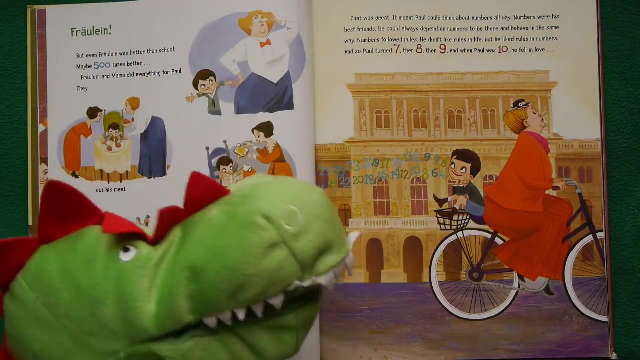 Yeah, they always are sick and coughing and picking their boogers and stuff. Yeah, they do. So she helped him solve his problem. Mama said he could stay home with Fraulein. Oh no, not Fraulein. 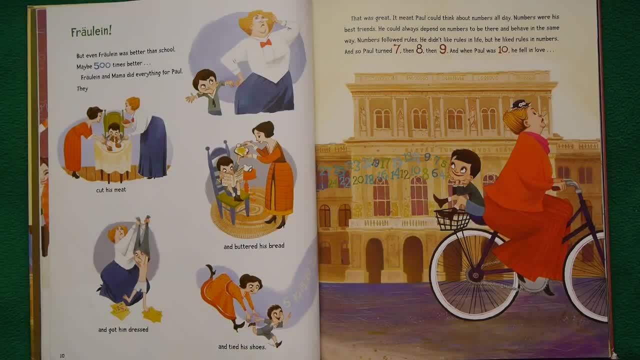 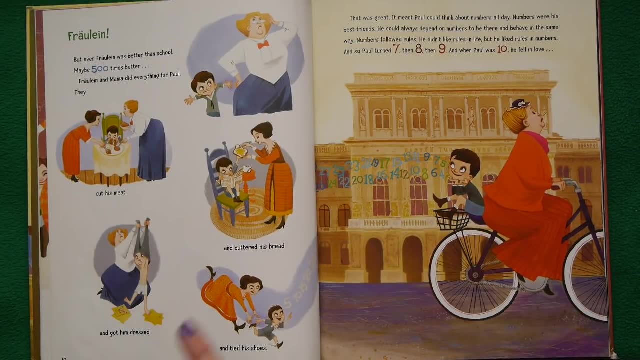 Well, even Fraulein was better than school, Maybe 500 times better. Fraulein and Mama did everything for Paul. They cut his meat and they littered his bread and got him dressed and tied his shoes, Oof. 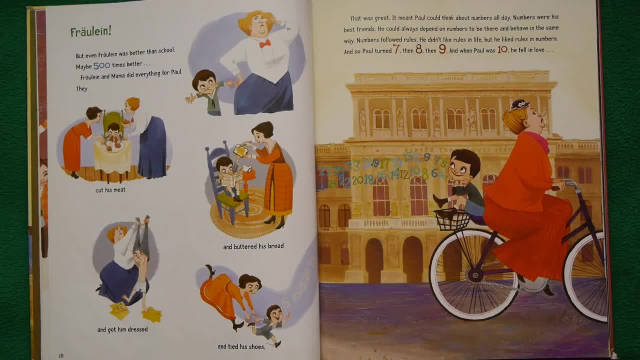 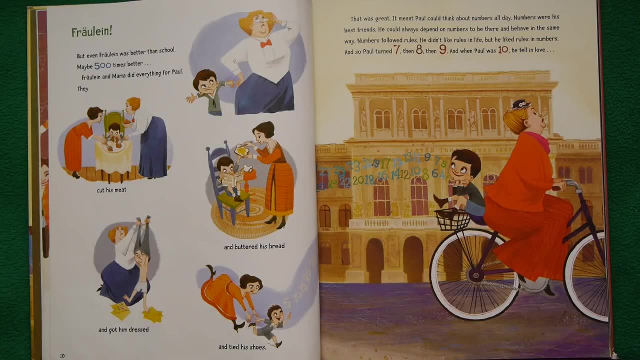 He's gonna be a little bit spoiled. That was great. It meant Paul could think about numbers all day. Numbers were his best friends. He could always depend on numbers to be there and behave in the same way. Numbers followed rules. Now, he didn't like rules in life. 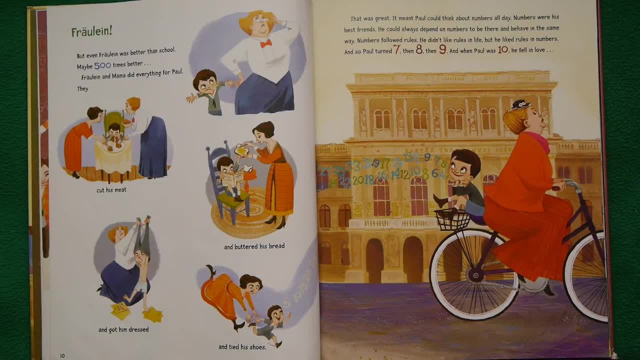 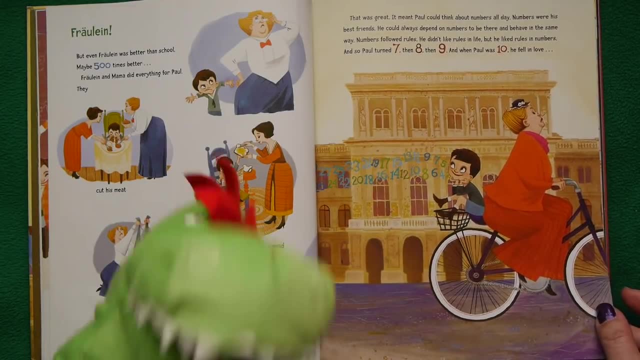 but he liked rules in numbers. And so Paul turned seven, then eight, then nine, and when Paul was ten he fell in love. What At ten. But that's so soon, I'm not ready. I'm not ready for a commitment. 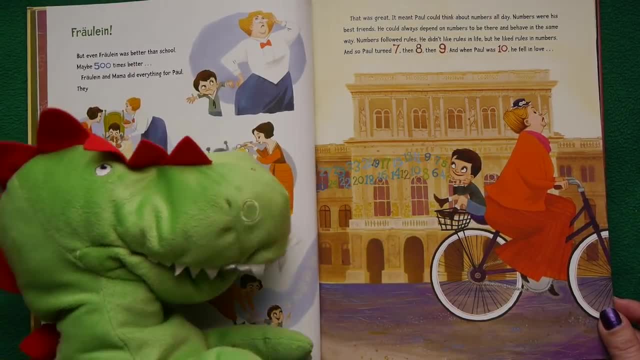 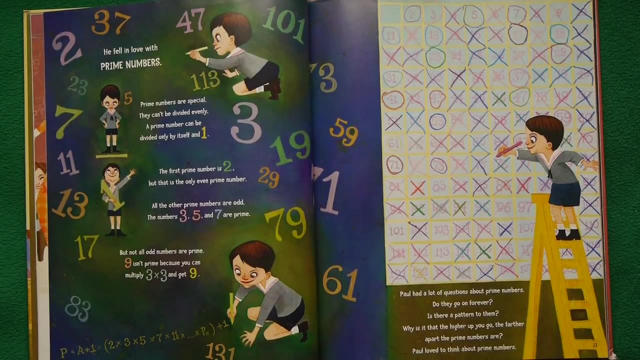 It's okay. This is Paul's story. You don't have to get a girlfriend yet. It looks like he's relieved. Okay, he fell in love with prime numbers. I thought it was gonna be a girl. Oh, this is much better, Okay. 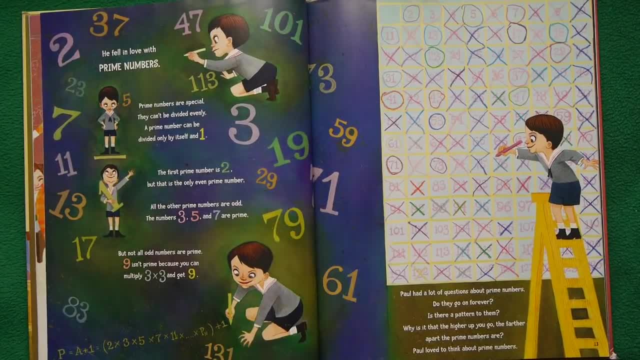 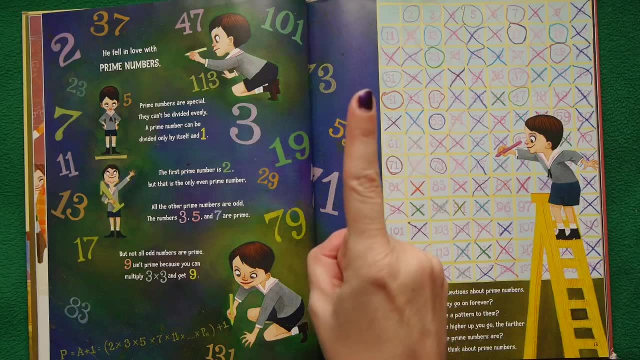 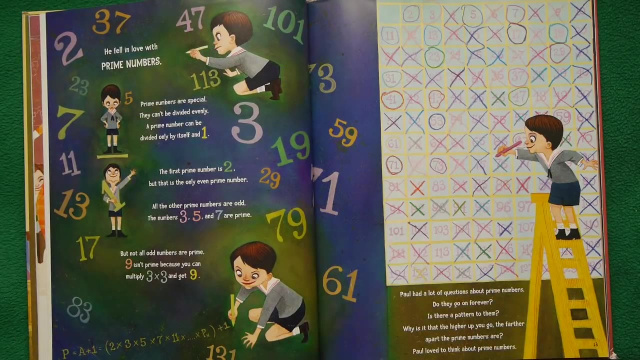 Alright, prime numbers. Prime numbers are special. They can't be divided evenly. A prime number can only be divided by itself and one. The first prime number is two, But that is the only the only even prime number. All the other prime numbers are odd. 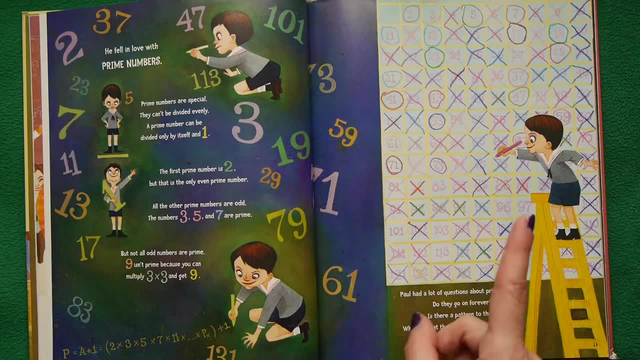 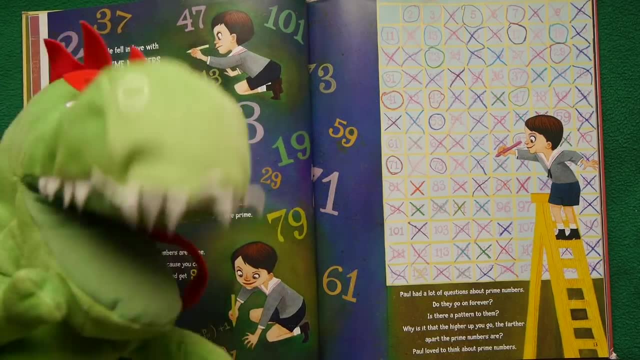 The numbers three, five and seven are prime, But not all odd numbers are prime. Nine isn't prime because you can multiply three times three and get nine. Are you following me? Yeah, yeah, I'm loving this. I really love math, so I really like this. 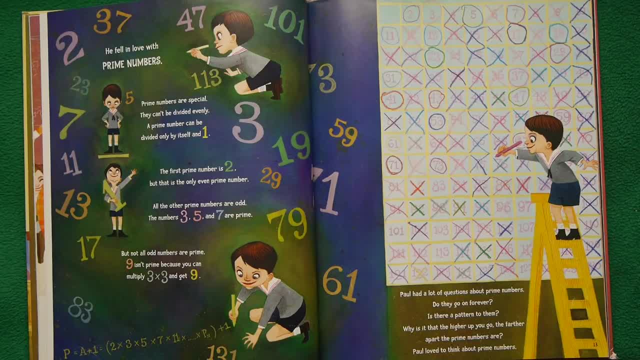 Okay, please keep going. Alright. Paul had a lot of questions about prime numbers. Do they go on forever? Is there a pattern to them? Why is it that the higher up you go, the farther apart the prime numbers are? Paul loved to think. 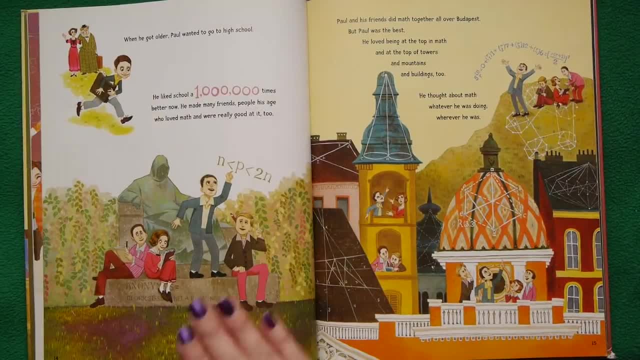 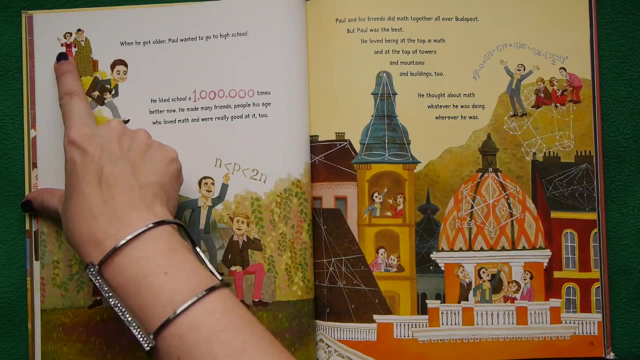 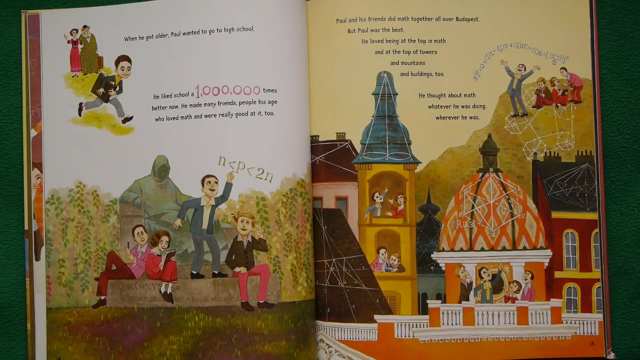 about prime numbers. When he got older, Paul actually wanted to go to high school. Oh, Fräulein, looks sad, Almost waving goodbye, also looking sad. He liked school a million times better now. He made friends, people his age. 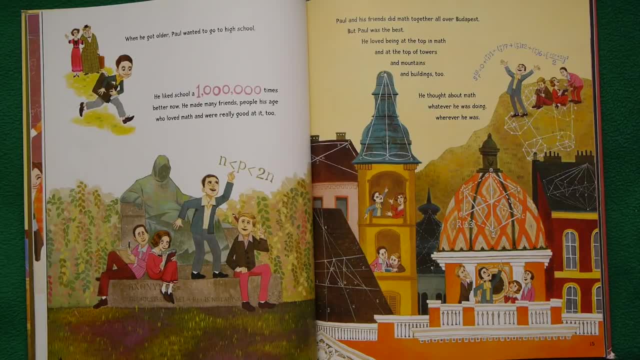 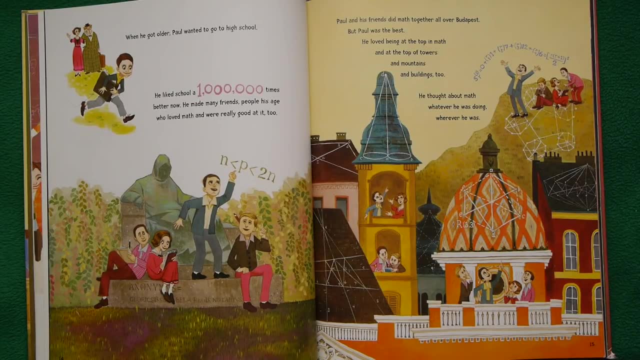 who loved math and were really good at it too. Now Paul and his friends did math together all over Budapest, But Paul was the best. He loved being at the top in math and at the top of towers and mountains and buildings too. He thought about math. 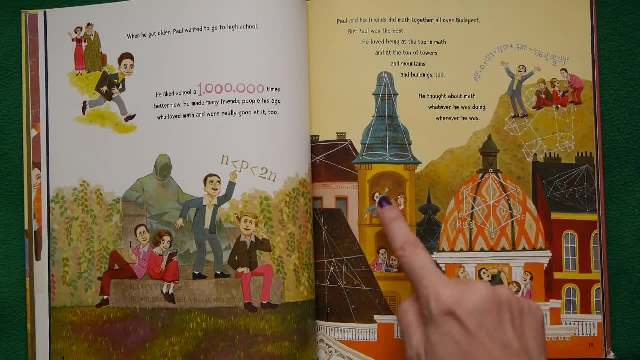 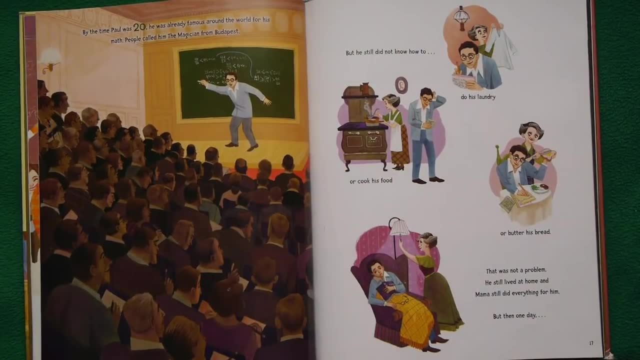 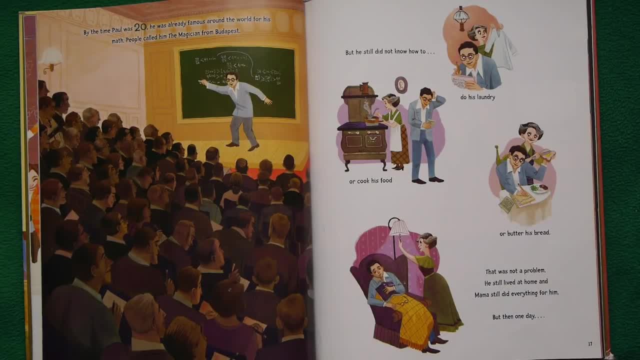 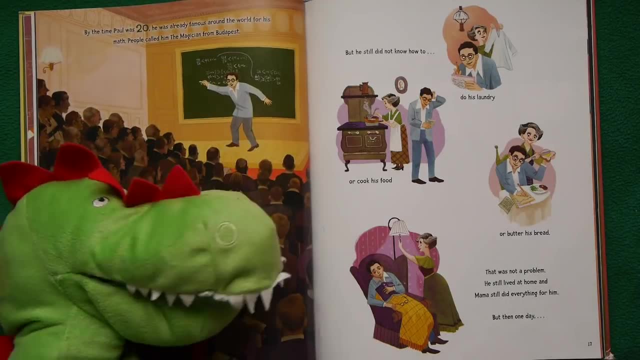 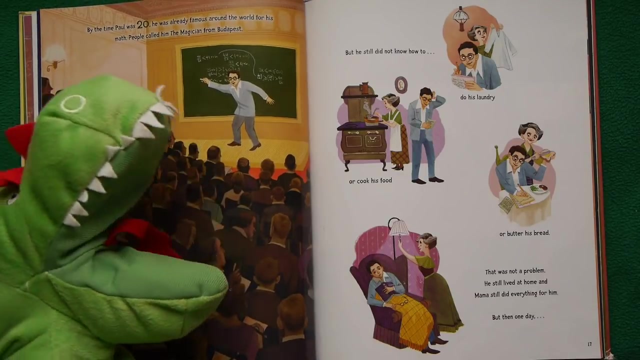 he was already famous around the world for his math. People called him the magician from Budapest. May I say something here? storyteller- Yes, Doug, What would you like to say? I just think I'm feeling very inspired right now because I see. 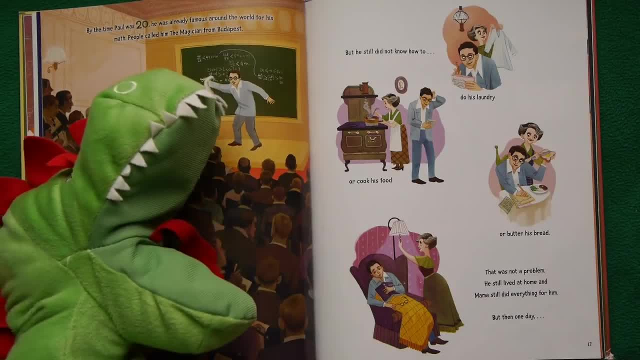 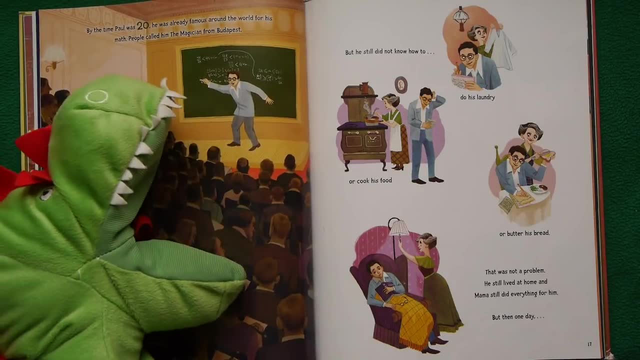 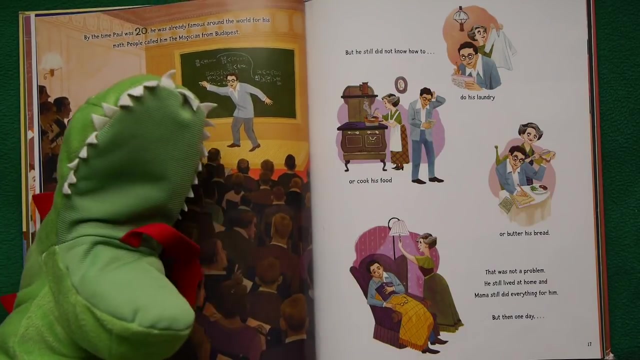 that even though Paul was a little kid, he still worked hard and really focused on his special talent. and look at that: it made him famous by 20.. By 20! That's really young to be famous for your math, isn't it? 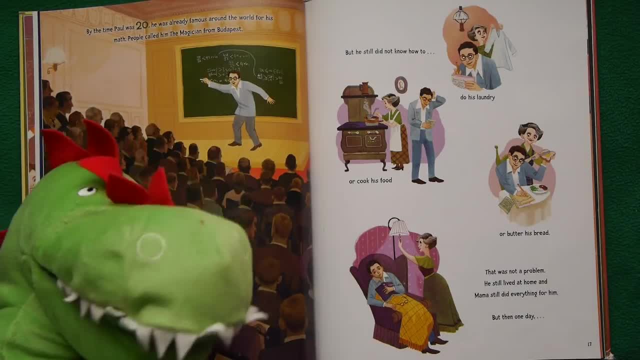 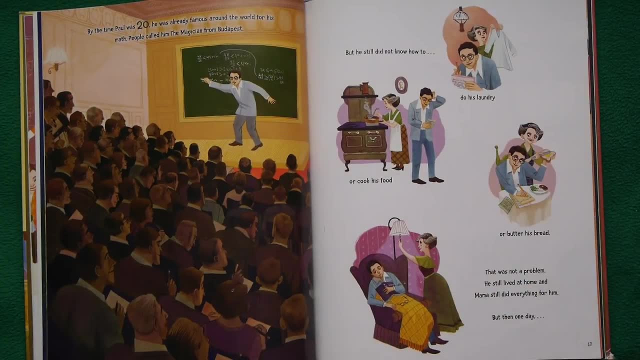 It is. Yeah, yeah, I'm very inspired to really work hard on my talents. Okay, there's more book, isn't there? Yes, But he still did not know how to do his laundry or cook his food or butter his bread. 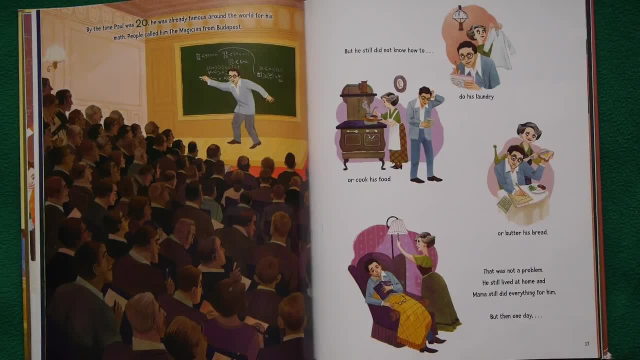 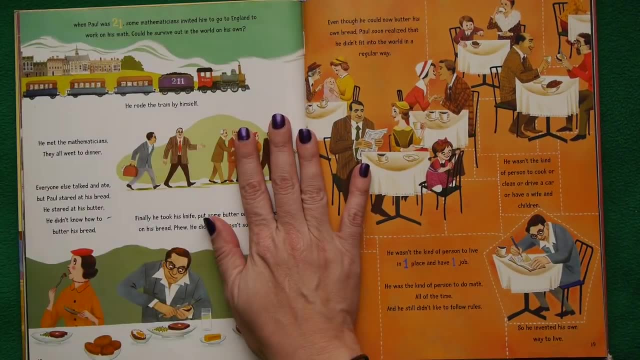 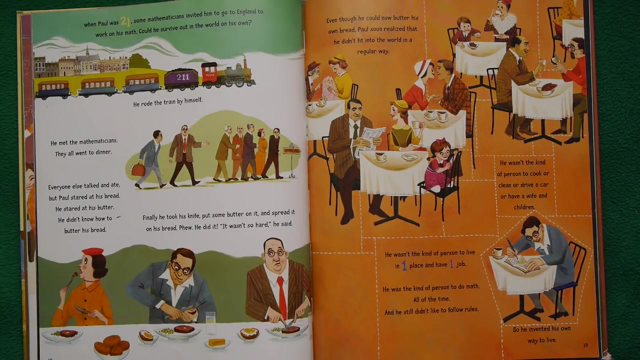 Hmm, I wonder why, But that was out of the problem. He still lived at home and Mama still did everything for him. But then one day, when Paul was 21,, some mathematicians invited him to go to England to work on his math. Could he survive? 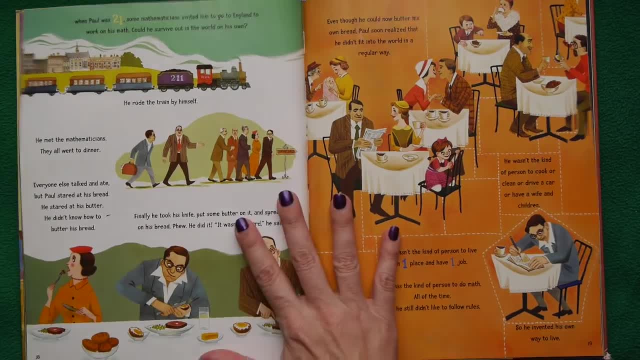 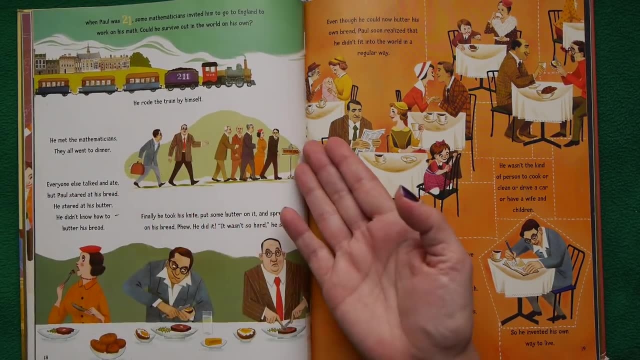 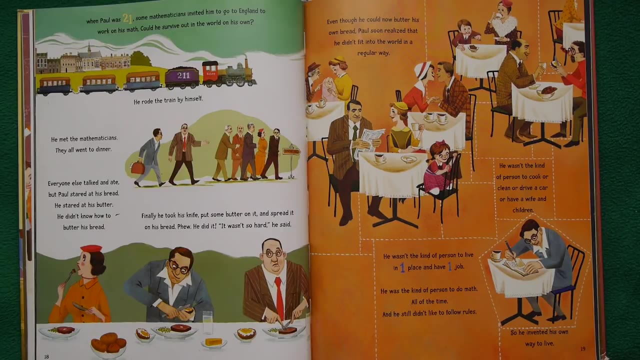 out in the world on his own. He rode the train by himself. He met the mathematicians. They all went to dinner. Everyone else talked and ate, But Paul stared at his bread. He stared at his butter. He did not know how to butter his bread. 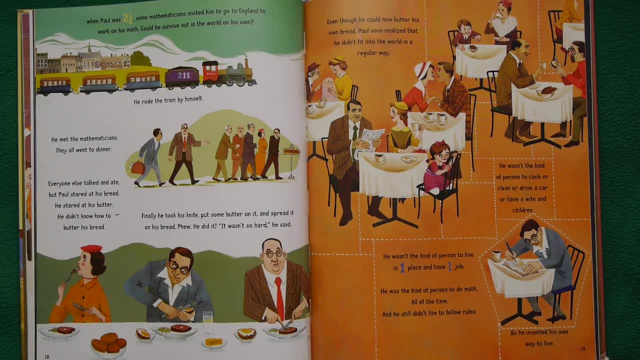 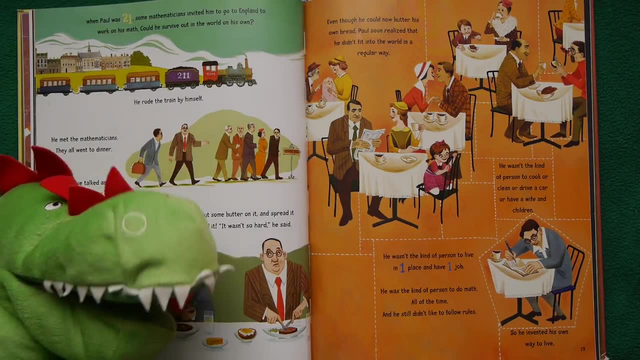 Huh. Finally, he took his knife, put some butter on it and spread it on his bread. He did it. It wasn't so hard, he said. Oh, that had me nervous. Well, even though he could now butter his own bread. 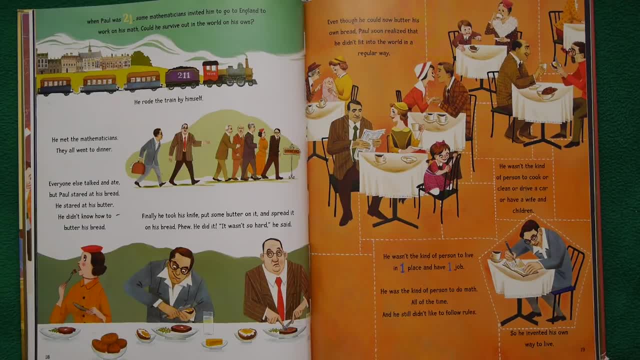 good boy, Paul, soon realized that he didn't fit into the world in a regular way. He wasn't the kind of person to cook or clean or drive a car or have a wife and children. He wasn't the kind of person to live in. 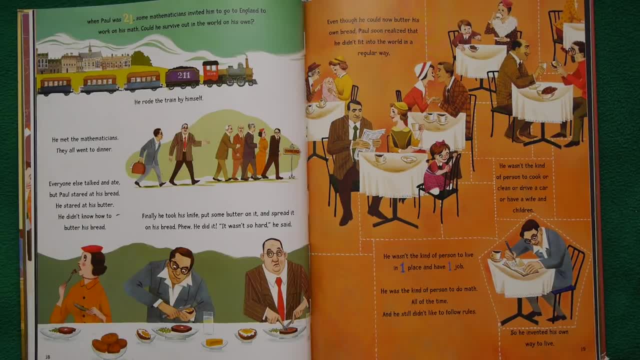 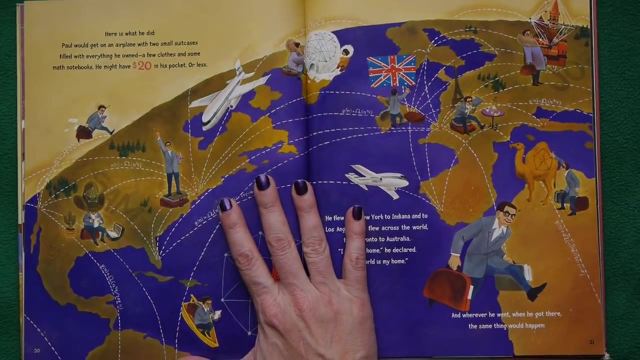 one place and have one job. He was the kind of person to do math all of the time And he still didn't like to follow rules, So he invented his own way to live. Did you know you could do that? You can invent your own way to live. 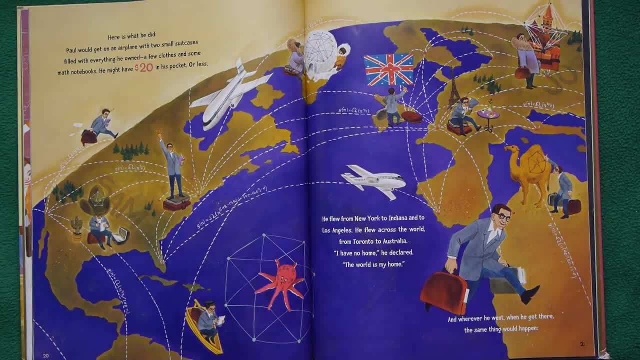 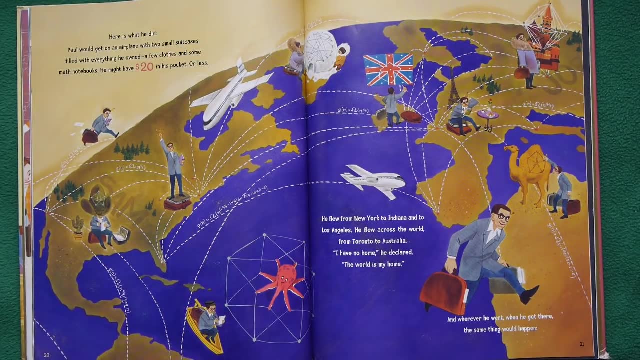 Here's what he did. Paul would get on an airplane with two small suitcases- One, two, one, two- And he would fill it with everything he owned: A few clothes, some math notebooks. He might have twenty dollars in his pocket. 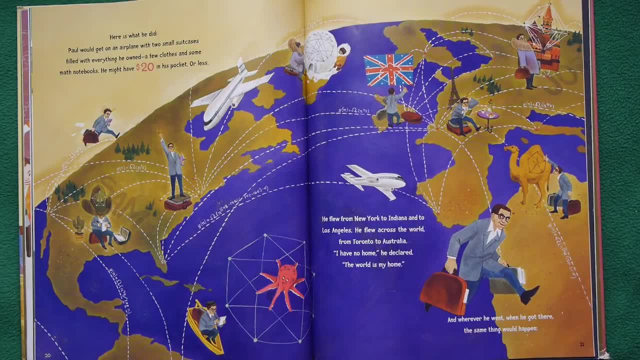 Or less. He flew from New York to Indiana and to Los Angeles. He flew across the world, from Toronto to Australia. I have no home, he declared. The world is my home And wherever he went when he got there, the 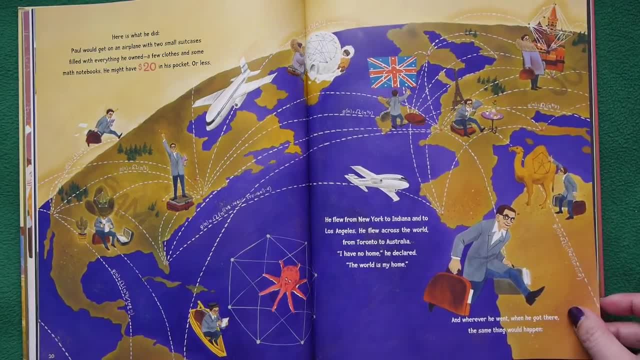 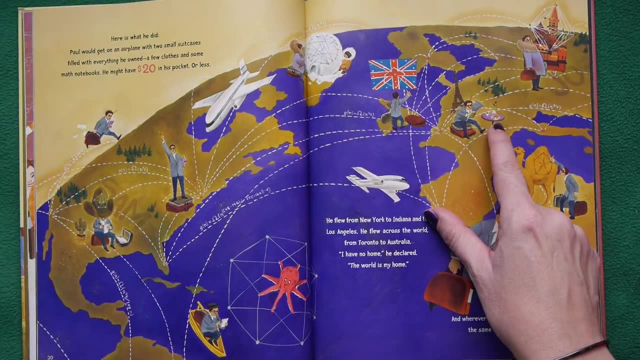 same thing would happen. I wonder what would happen. But before I turn the page I just wanted to enjoy this. Look at that. There he is in an igloo in Alaska. There he is in merry old England. Here he is enjoying a croissant. 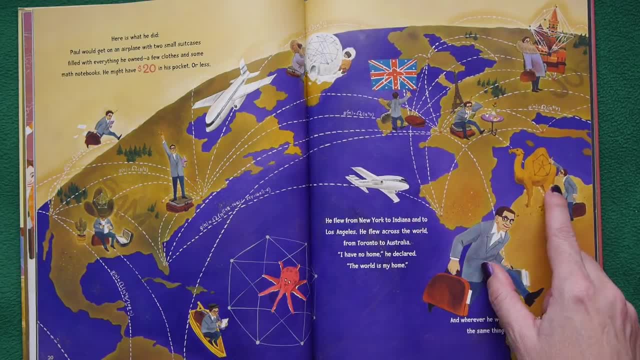 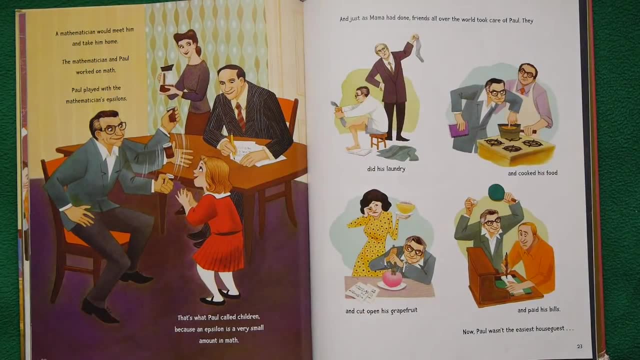 and a cafe au lait by the Eiffel Tower. Here he is on a camel. Hey Got to some interesting places. Every time he would go somewhere, a mathematician would meet him and take him home. Why? Because, of course, he's famous. 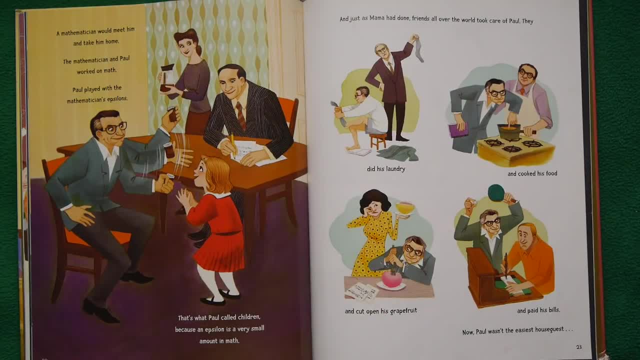 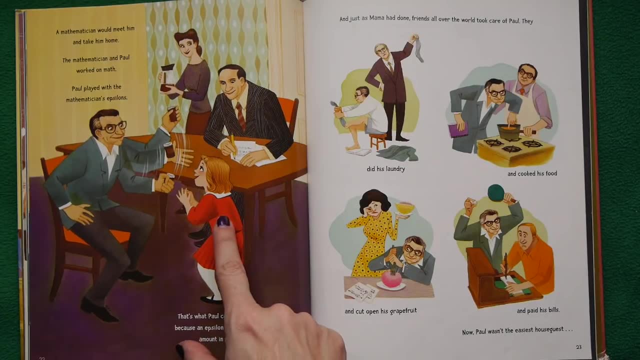 And other mathematicians want to meet a famous mathematician, So the mathematician and Paul would work on math. Paul played with the mathematician's epsilons- That was Paul's special word for little kids- Epsilons- Because an epsilon is a very small. 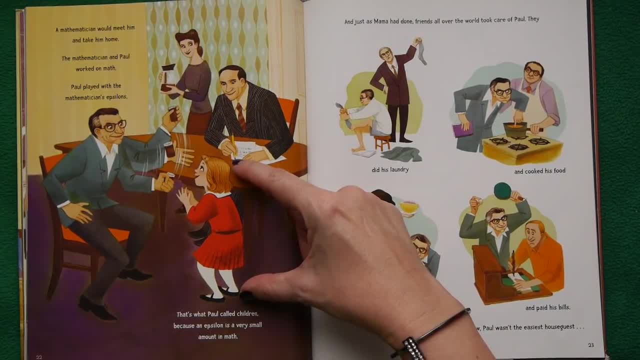 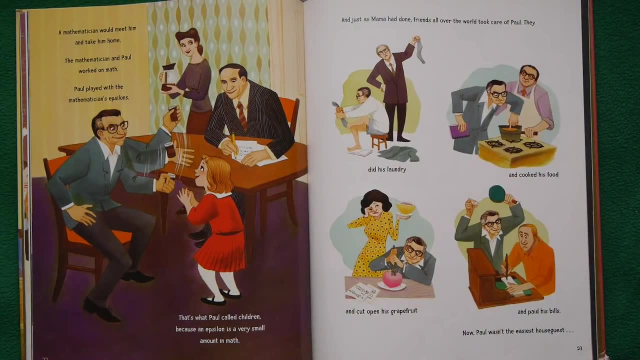 amount in math. Get it A little small amount in math is like a math joke. I like math jokes. So, just as Mama had done, friends all over the world took care of Paul. They did his laundry and cooked his food and 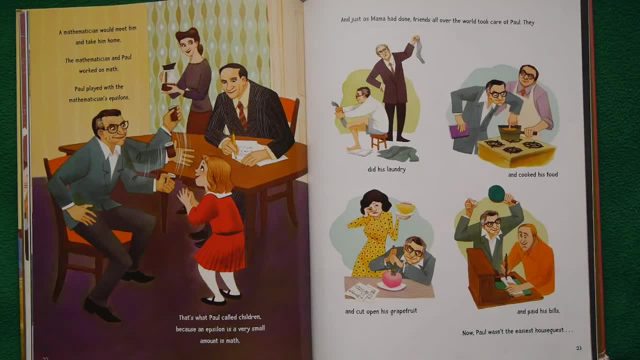 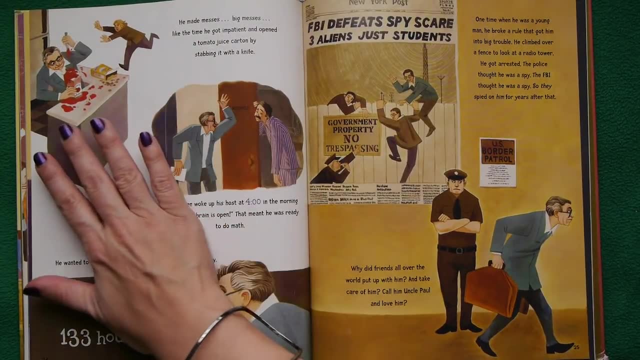 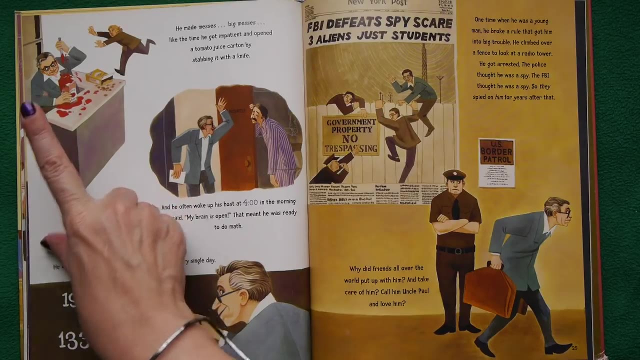 cut open his grapefruit and paid his bills. Now, Paul wasn't the easiest house guest. He made messes, Big messes, Like the time he got impatient and opened a tomato juice carton by stabbing it with a knife, And he often woke up his host at four. 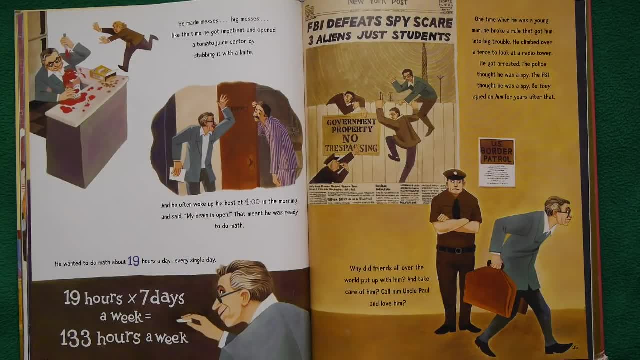 in the morning and said: My brain is open. That meant he was ready to do math. He wanted to do math about 19 hours a day, every single day. Now, that is single-minded passion. 21 hours, 7 days a week equals. 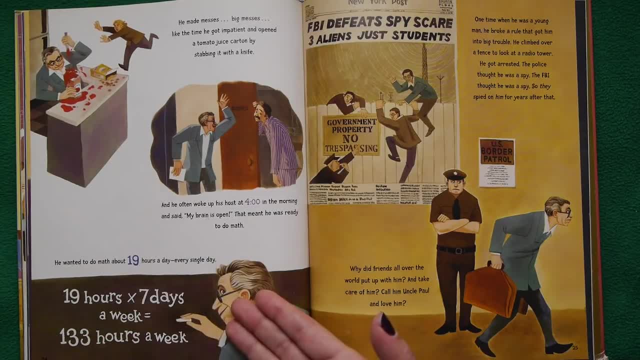 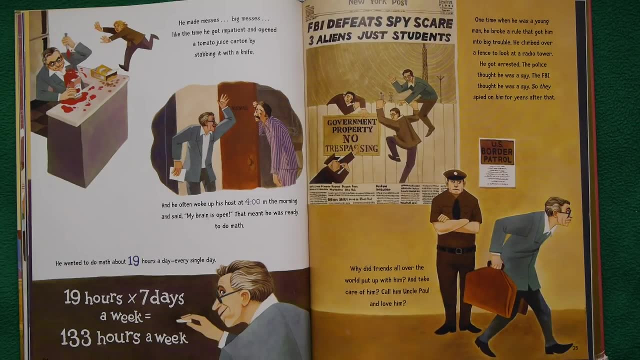 133 hours a week, So you can imagine how much calculating he got accomplished. One time, when he was a young man, he broke a rule that got him into big trouble. He climbed over a fence to look at a radio tower. He got arrested. The police, 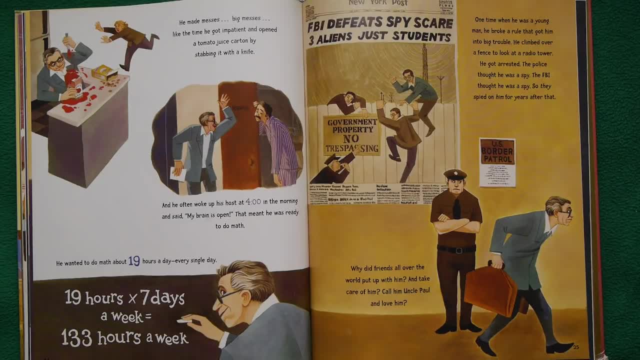 thought he was a spy. The FBI thought he was a spy, So they spied on him for years after that. Now, why did friends all over the world put up with Paul and take care of him, Call him Uncle Paul and love him? Why? Why? 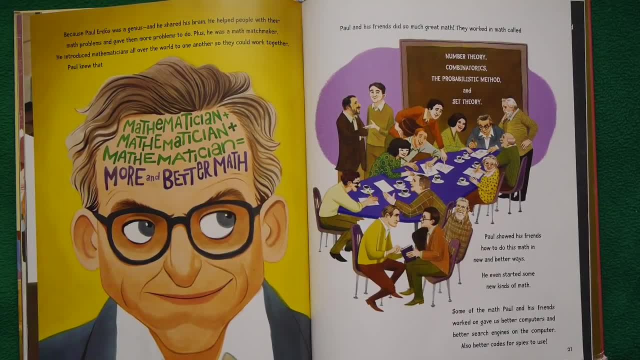 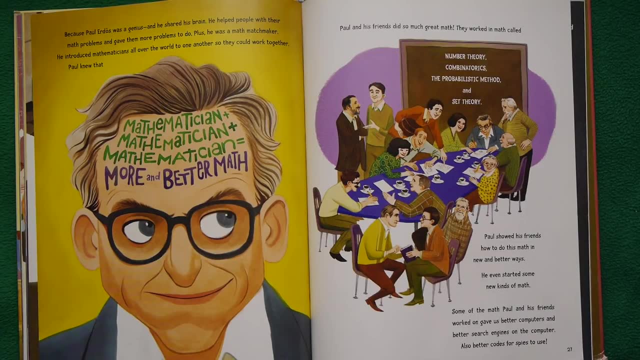 Why do you think? Why do you think? Because Paul Erdős was a genius And he shared his brain. He helped people with their math problems and gave them more problems to do. That means he was challenging them to be even better and smarter. 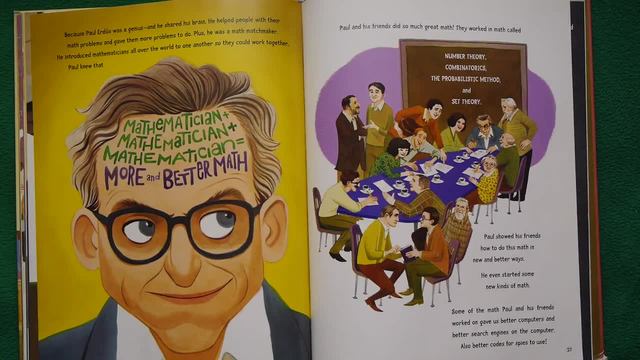 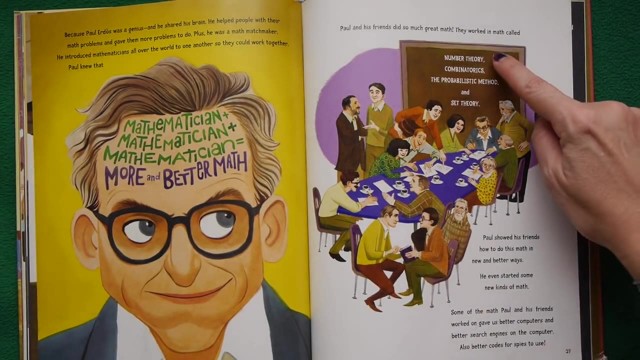 Plus, he was a math matchmaker. He introduced mathematicians all over the world to one another so they could work together. And Paul, he knew that Paul and his friends did so much great math. They worked in math called number theory, combinatorics. 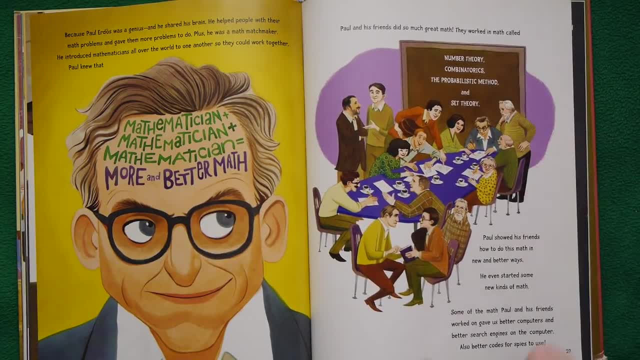 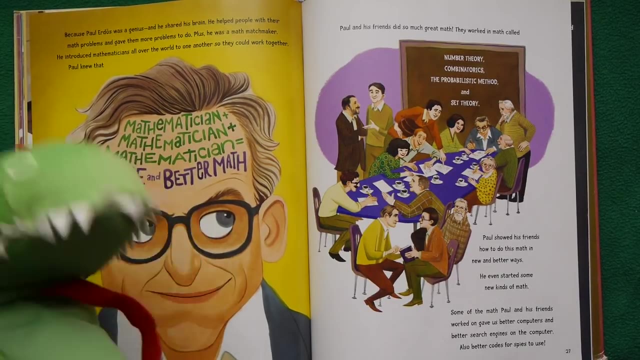 the probabilistic method and set theory. Paul showed his friends how to do this math in new and better ways. He even started some new kinds of math. Some of the math that Paul and his friends worked on gave us better computers, Computers. So it affected today. 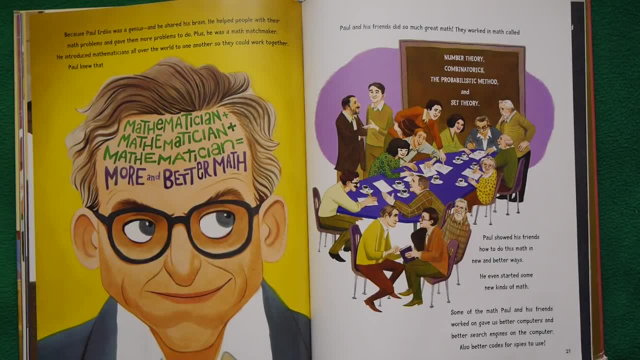 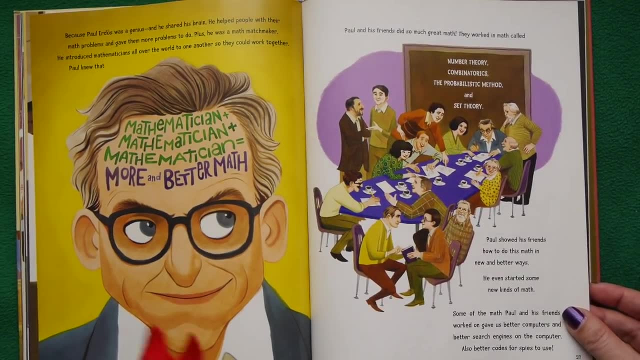 even though he started a long time ago Exactly. And better search engines like Google on the computer. Also better codes for spies to use. Oh, that's funny, because they thought he was a spy, But he wasn't. He was just a. 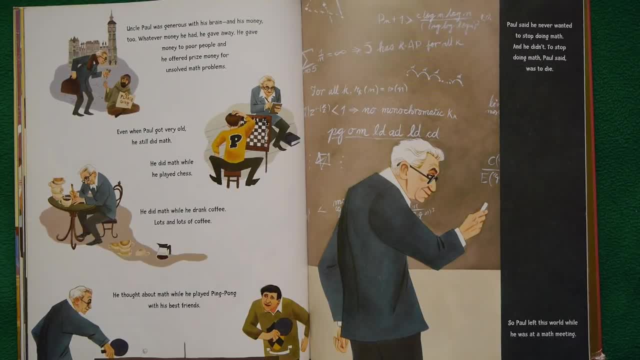 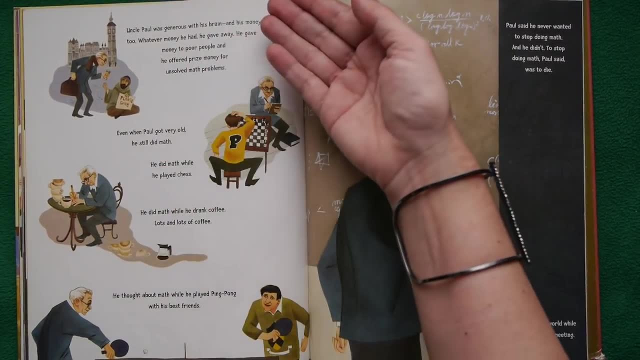 brilliant math guy. Uncle Paul, was generous with his brain, And people love generosity. Yes, they love things that make them smarter and stronger and better. And he was generous with his money too. Wherever money he had, he gave away. He gave money to poor people. 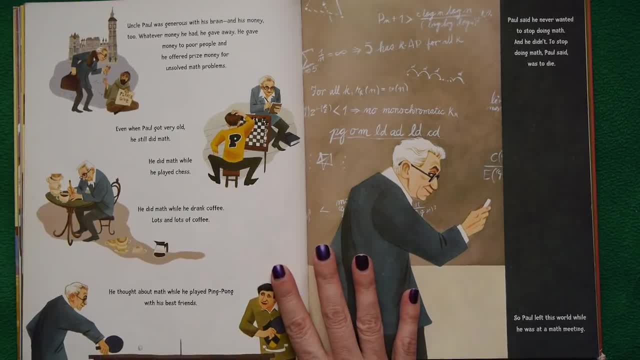 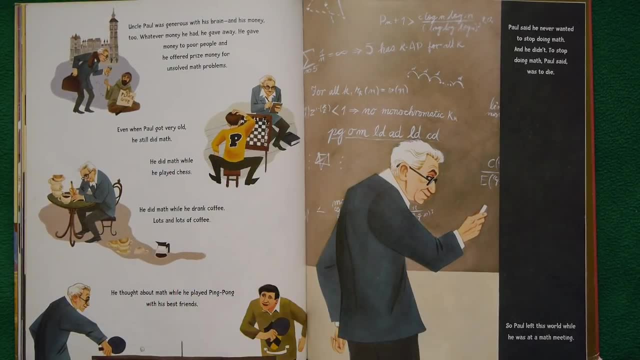 and he offered prize money for unsolved math problems, Which is a great way to inspire people to do more math. Even when Paul got very old, he still did math. He did math while he played chess, He did math while he drank coffee. Lots and lots. 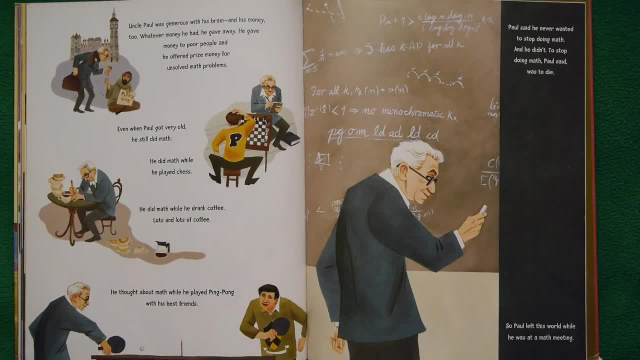 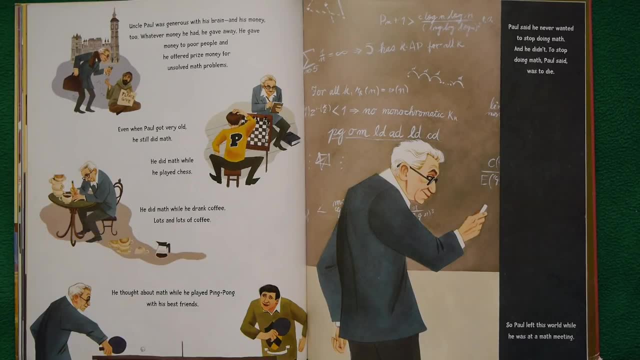 of coffee. He thought about math while he played ping pong with his best friends. Paul said he never wanted to stop doing math And he didn't. To stop doing math, Paul said, was to die. So Paul left this world while he was. 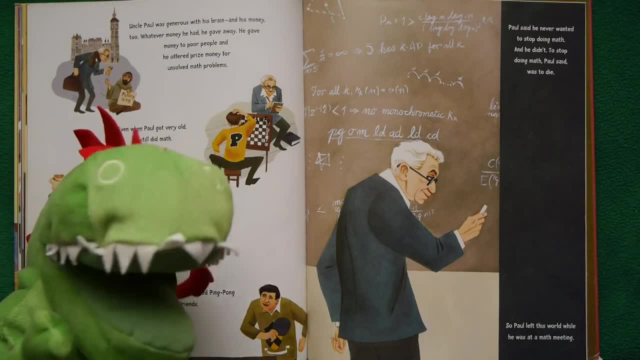 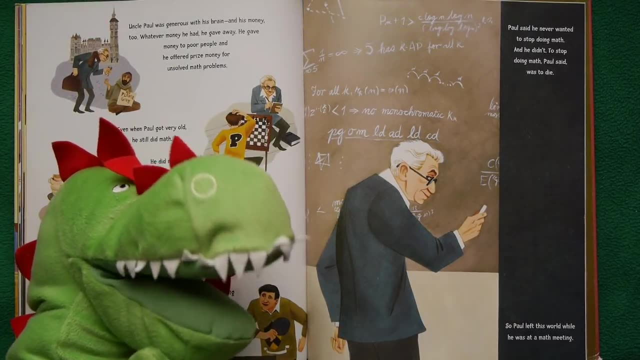 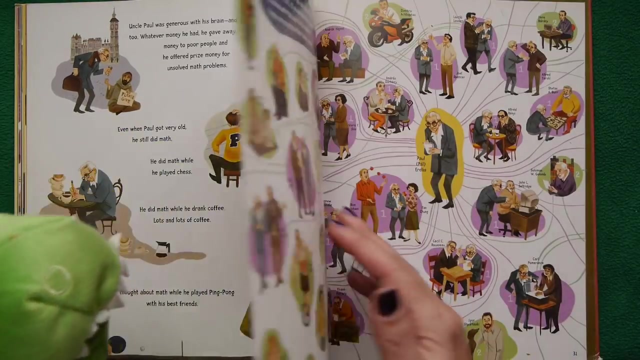 at a math meeting. So he never stopped. Wow, That's incredible. He never lost his passion And he never gave it up, And he devoted his whole life to it. Exactly All over the world mathematicians still talk about and love Uncle Paul. 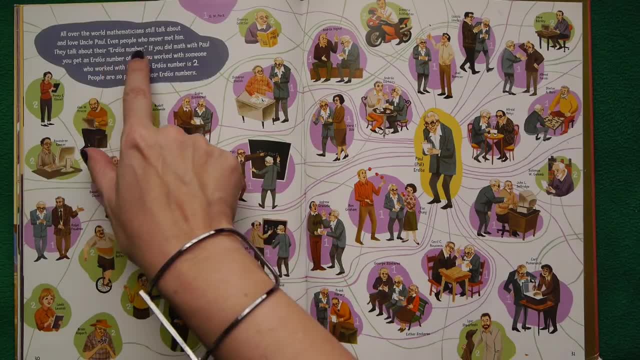 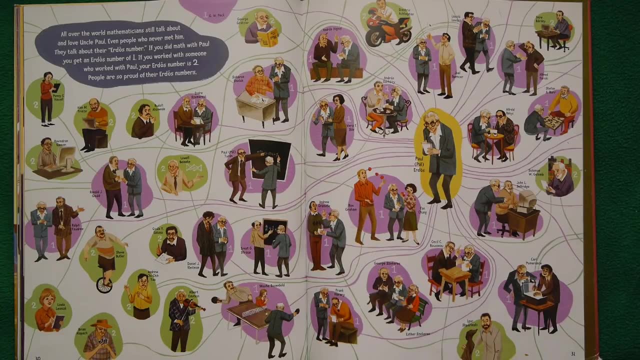 Even people who never met him. They talk about their number. If you did math with Paul, you get an Erdős number of 1. If you worked with someone who worked with Paul, your Erdős number is 2.. People are so. 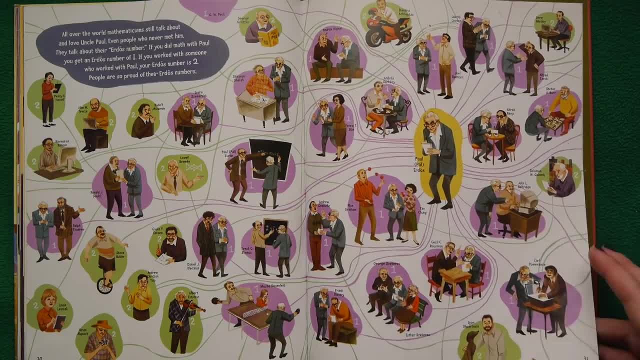 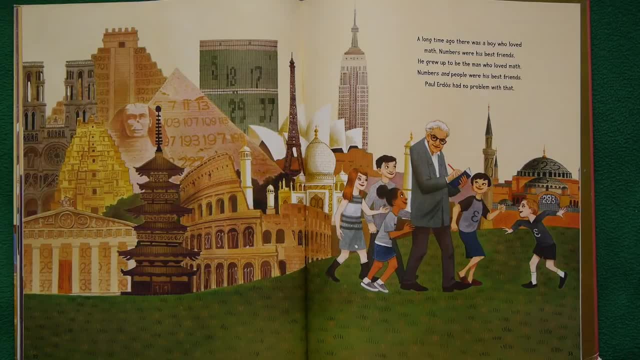 proud of their Erdős numbers. That's sort of like 9 degrees of Kevin Bacon. but in math, A long time ago, there was a boy who loved math. Numbers were his best friends. He grew up to be the man who loved math. 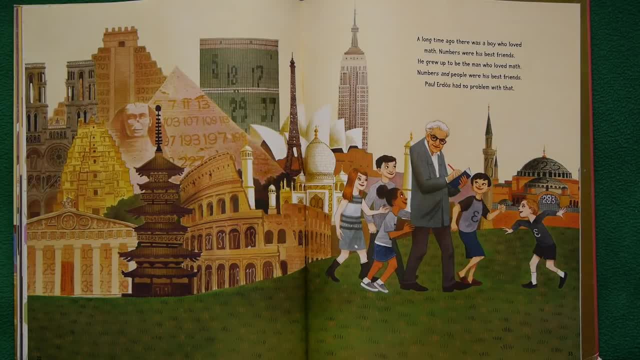 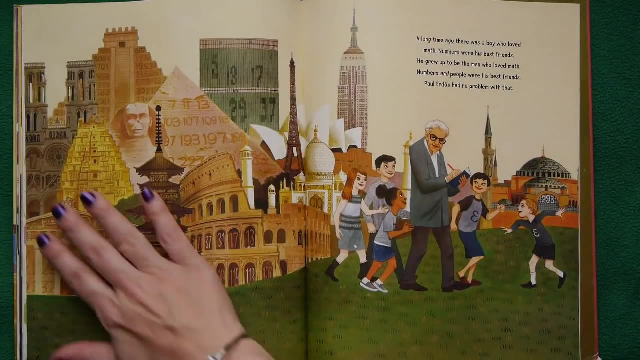 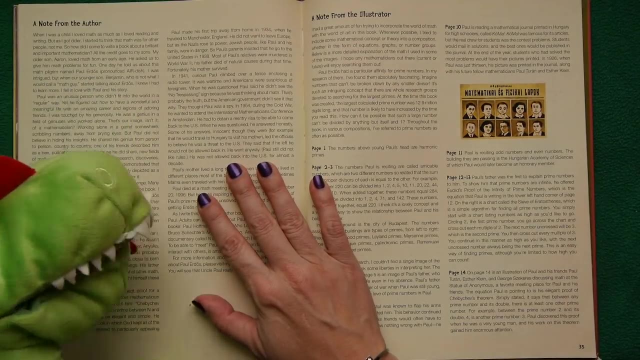 Numbers and people were his best friends. Paul Erdős had no problem with that. There he is with the little epsilons. All over the world he traveled doing what he loved. Wow, That's a lot of notes from the author. 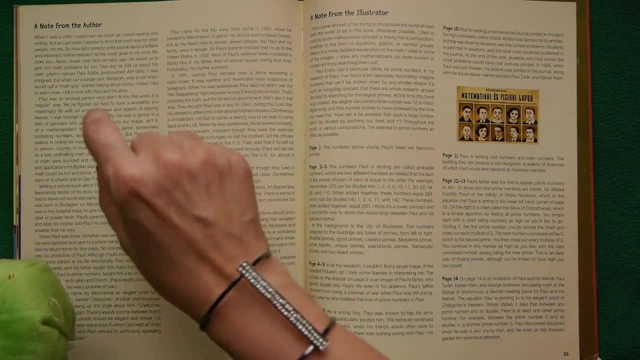 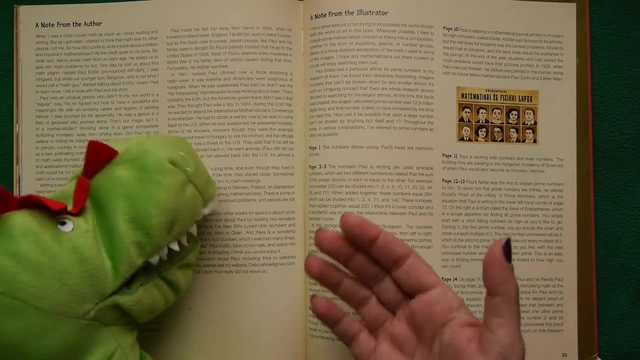 Yes, there are, But let me give you just a few quick more facts to take with you, because this Paul Erdős fellow- he would make a phenomenal book report, Don't you think? Oh yeah, That's very interesting. People don't really. 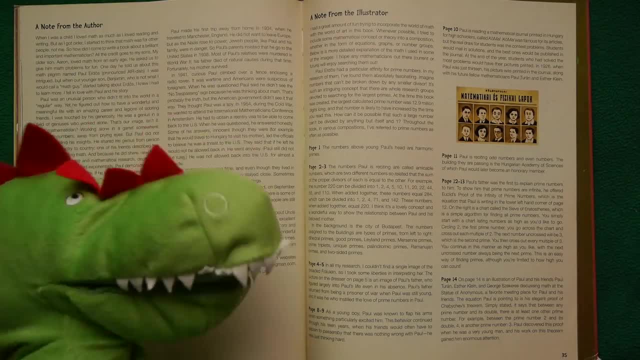 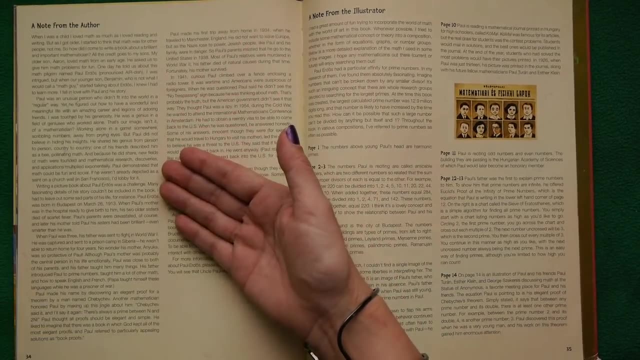 know much about him And if you love math, like I do, he's very inspirational. Yeah, exactly, It turns out he was. of course we mentioned he was born in Budapest. It was his father who taught him a lot about math. Yeah, yeah. 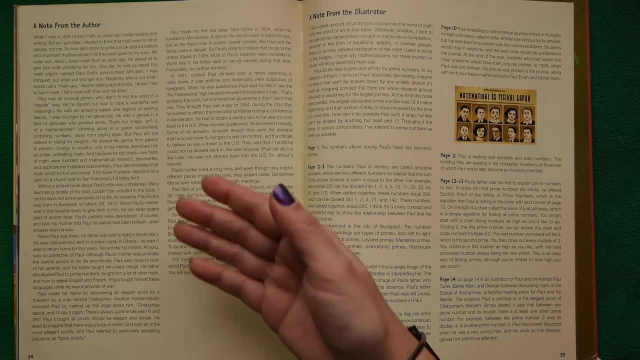 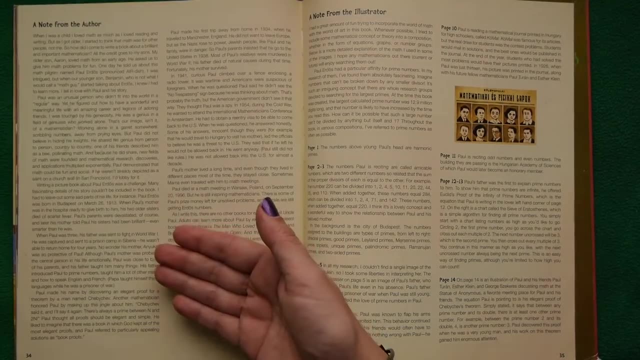 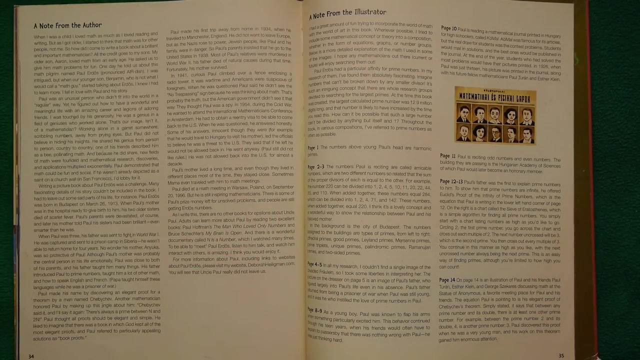 And his mother as well. Yeah, she was a teacher, And his father also taught him how to speak English and French. And his dad was smart as well, because the dad was a prisoner of war, And he taught himself how to speak English and French while he was a prisoner. And then 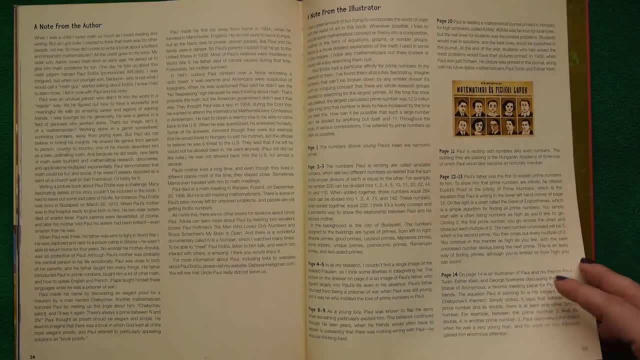 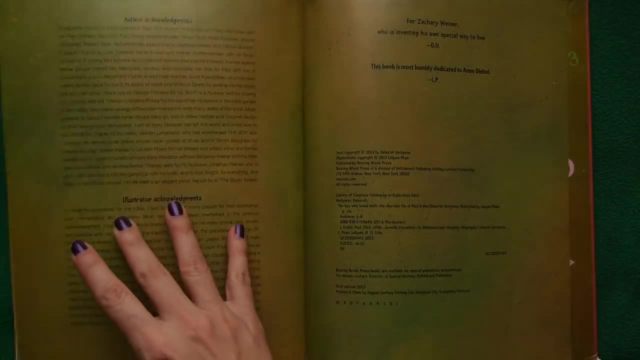 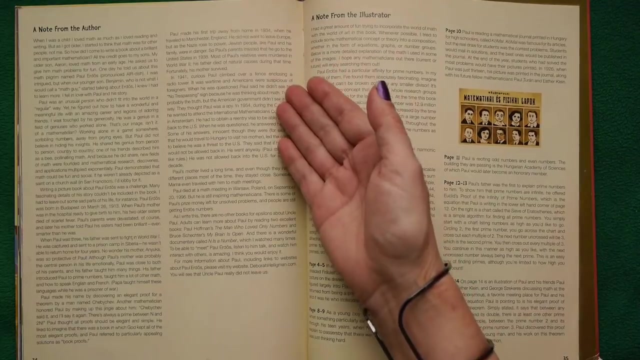 went on and taught his son And then, if you get this book for yourself- which I highly recommend because it's full of great, great interesting detail and facts about him- You know you can learn so much more detail about his life and about when they thought. 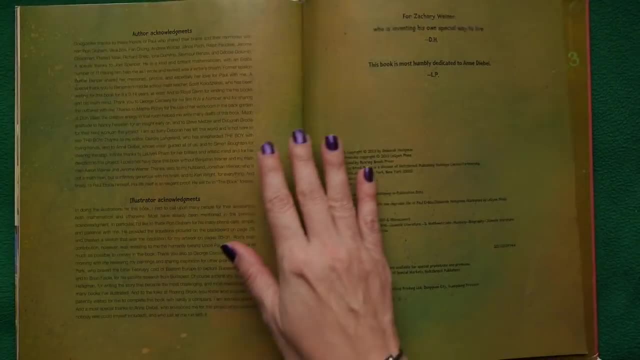 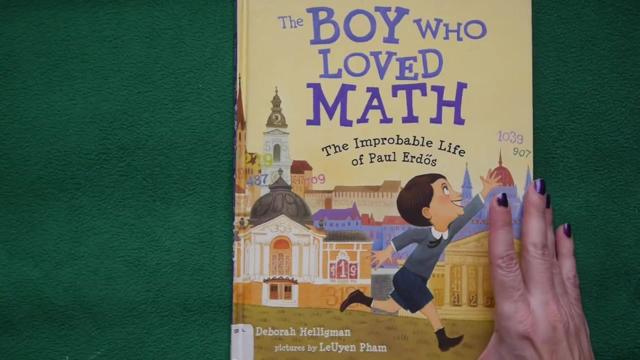 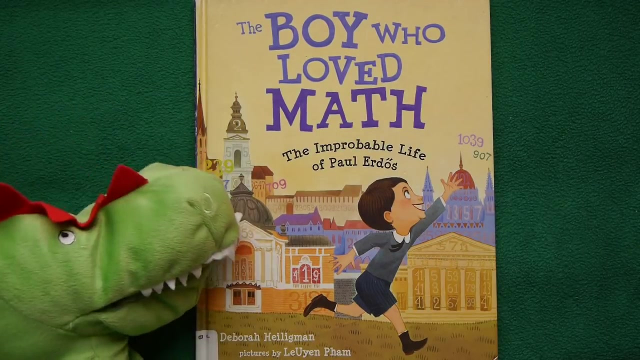 he was a spy. I mean just great stuff. And, by the way, the author of this book actually interviewed people who knew him growing up, knew him as a younger man, knew him as a older man, So he got first-hand information. 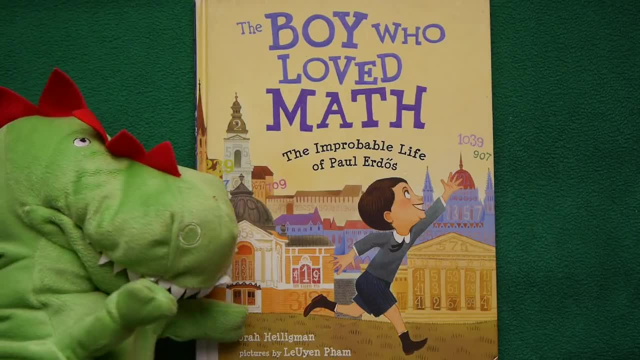 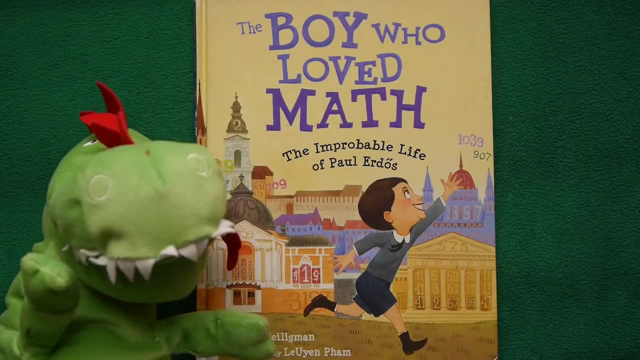 about him so that the book would be accurate Exactly So. it's not a pretend book, It's not make-believe, No, it's actually a real story. Well kid, I hope that you enjoyed The Boy Who Loved Math as much as. 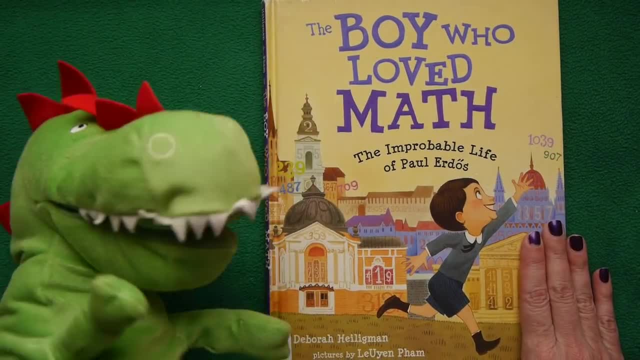 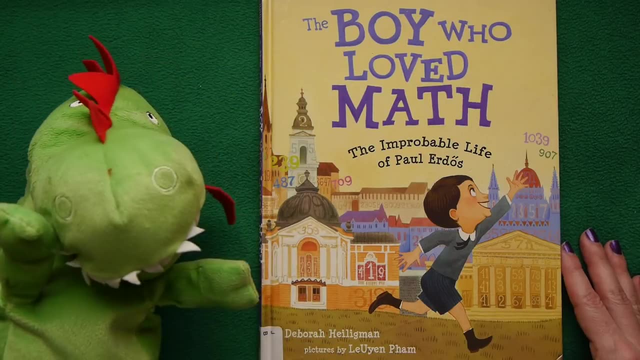 I do. Oh, wow, I really think that it's inspiring. And also I would like to say that it's not just inspiring for people who love math. Oh, it's also inspiring for people who love anything. to see that, if you. 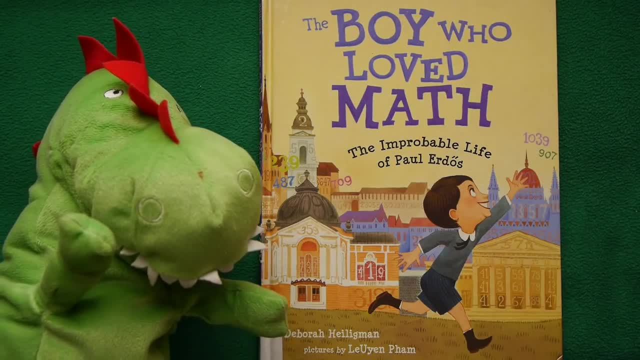 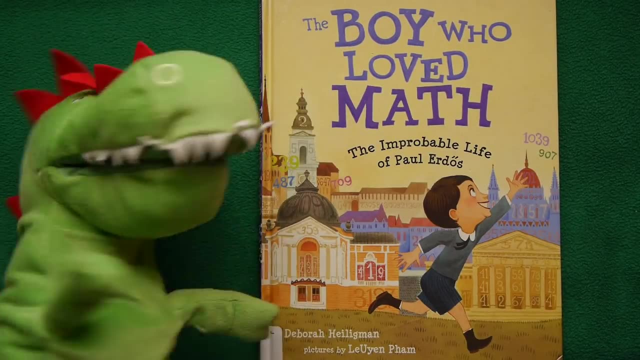 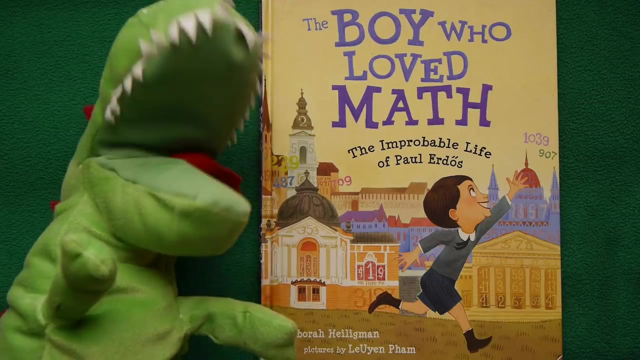 follow your passion and create your own way, you can do great things with your life. That's great. That's true, Because if, like you're good at something else, like science or drawing or dancing or writing, if you dedicate a lot of time and 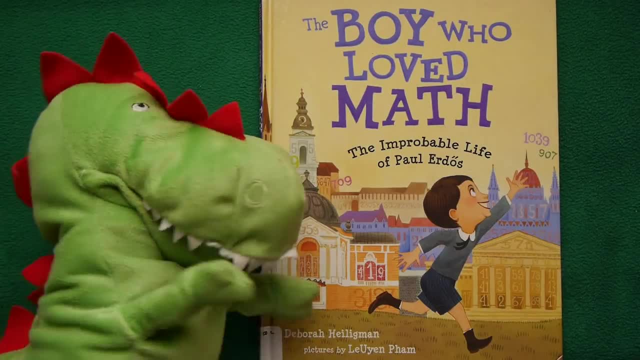 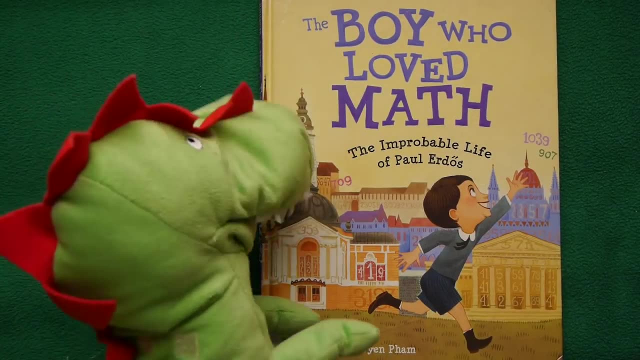 passion and energy to it, you can do great things Exactly. Thanks, kid, for joining us on this incredibly educational channel. Hit it Kid time, Story time. I love this book. Can I keep it?